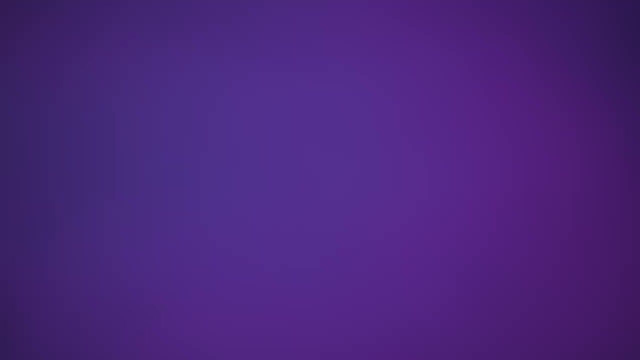 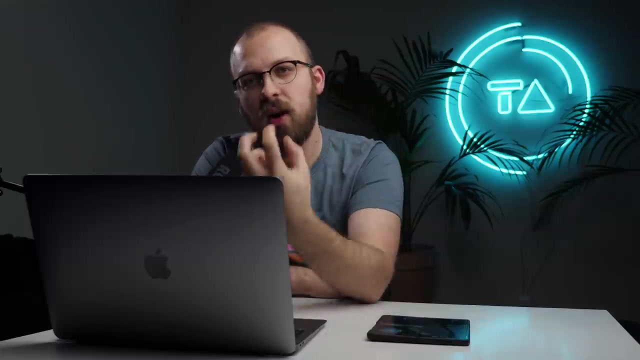 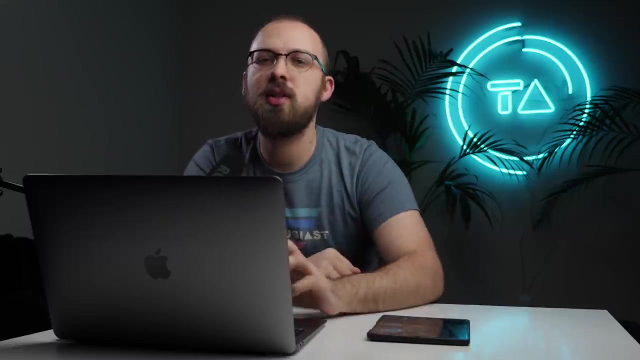 is very solid according to many different metrics. Their phone sales are off the roof. Their ecosystem products- so AirPods, Apple Watches, iPads, all the things that surround the iPhone very strong and thick. They're creating this sort of walled garden very effectively to keep you in the ecosystem. Their 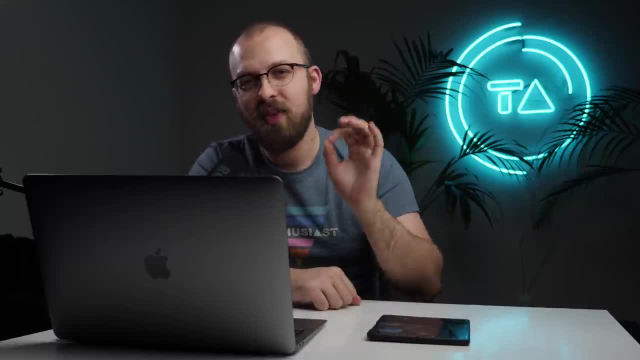 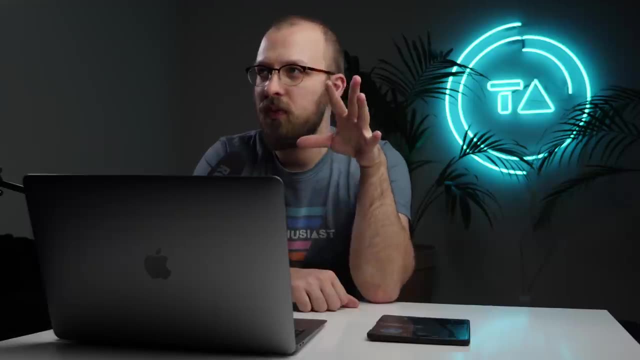 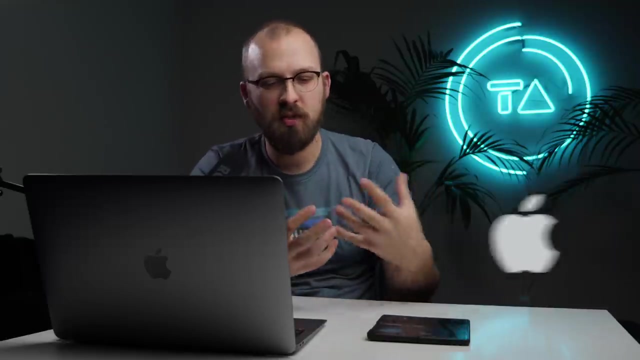 services business is going incredibly strong as well. Their key technologies, such as the A-series chips, are as competitive as they have ever been. There were, I guess, challenges to their business in terms of regulatory pressure, whether they have to change their business in any significant way. 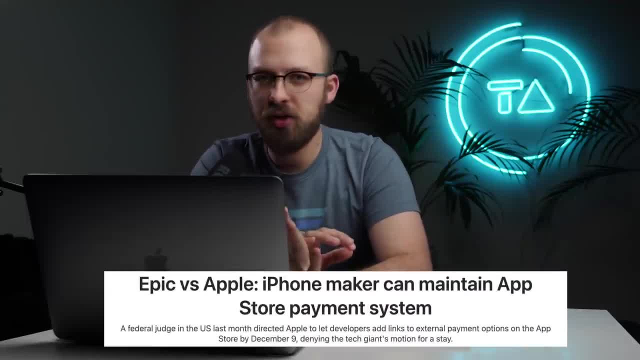 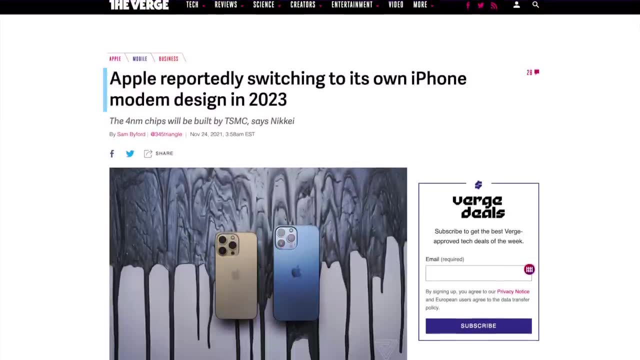 But basically Apple got out of all of those regulatory challenges more or less unharmed: The Epic trial, everything else, Basically nothing hurt their business. They have a strong outlook. They're going to be making their own 5G modem soon. foldable iPhone soon, Apple glasses. 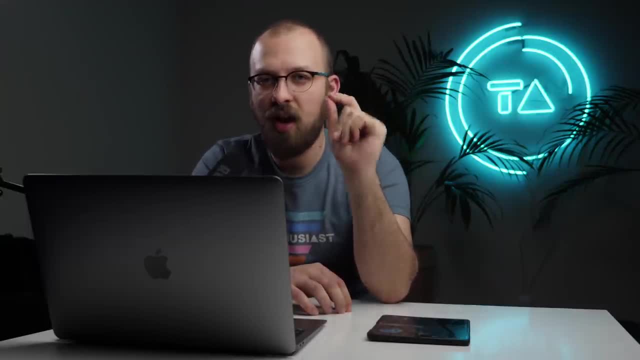 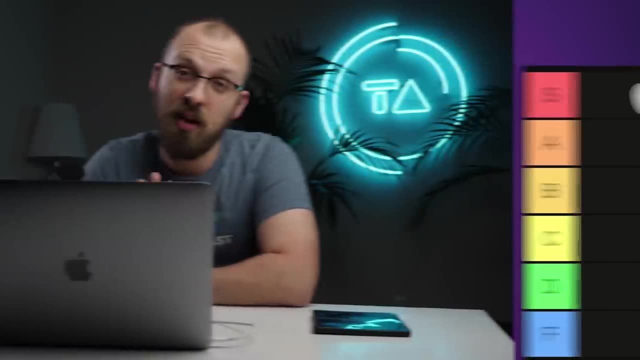 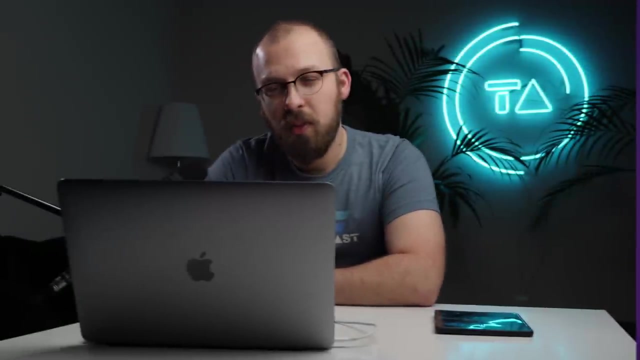 who knows what. I think this is a company that is in a clear S-tier, and they're doing a very solid job, even if I myself am not choosing to use their products. Asus, I would put this into the D-tier. They always have promising phones, In fact. 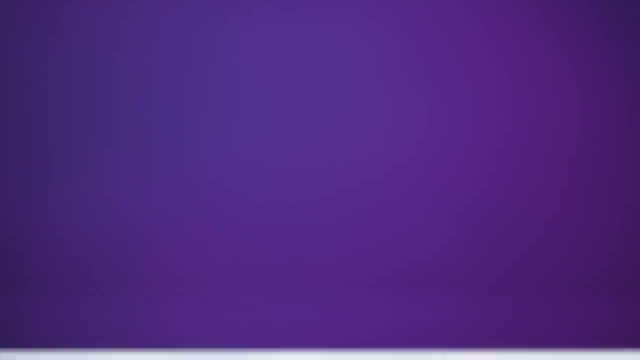 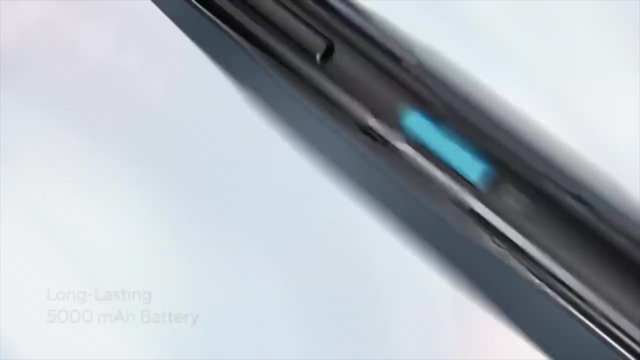 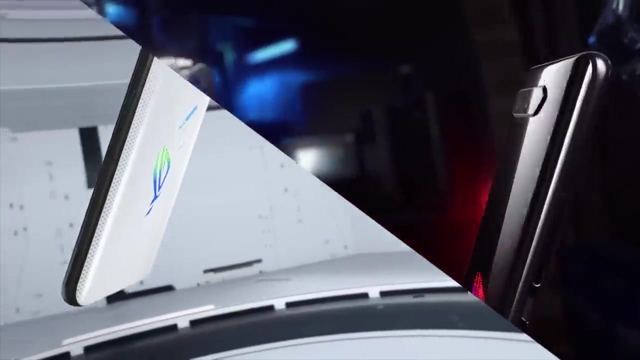 they had three promising phones this year. They had the flip style Zenfone 8, I think. Then they had the regular compact Zenfone 8, one of the only compact Android flagships, And of course, their ROG phone series as well. They're always promising, They look good And then they basically. 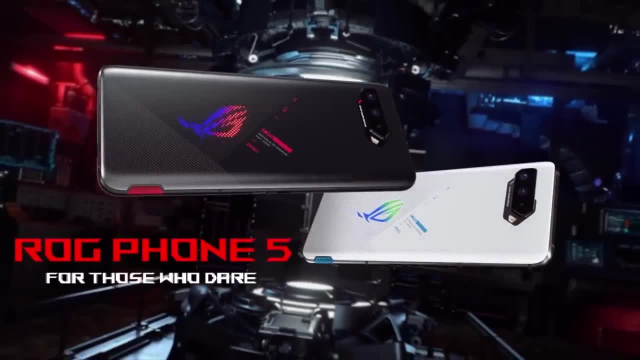 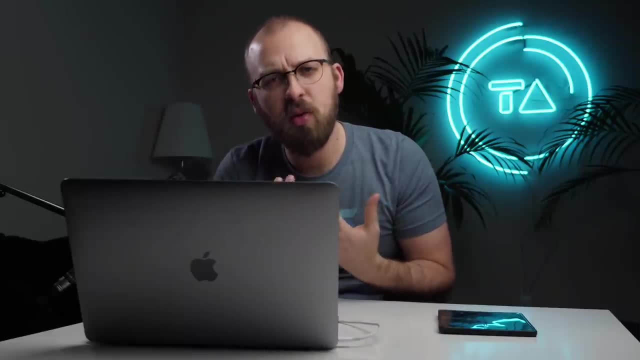 never sell because Asus doesn't do any marketing and they're barely available anywhere at all. I had a friend who wanted to have a compact Android phone. It took me, I think, almost a week to remember that the Asus Zenfone 8 even exists, and then he could barely buy it. So the only stats that I could find of 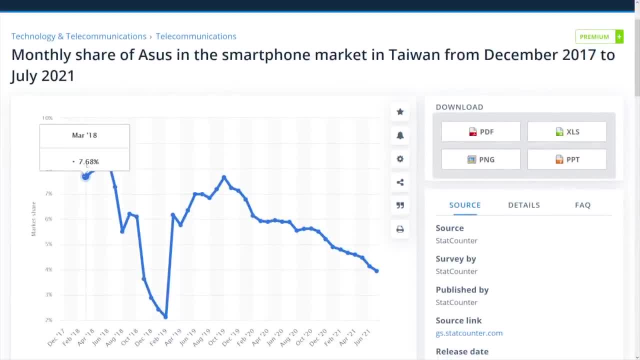 this company was that in Taiwan, according to StatCounter, which is not a very reliable source at all, but apparently that's their strongest market and their market share is declining. It went from about 5% to about 4% in the last year or so, I don't know. Interesting products. 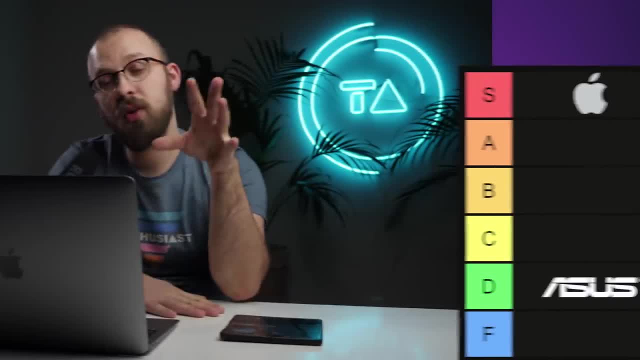 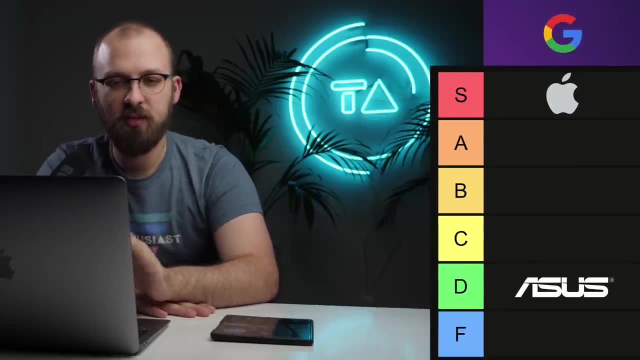 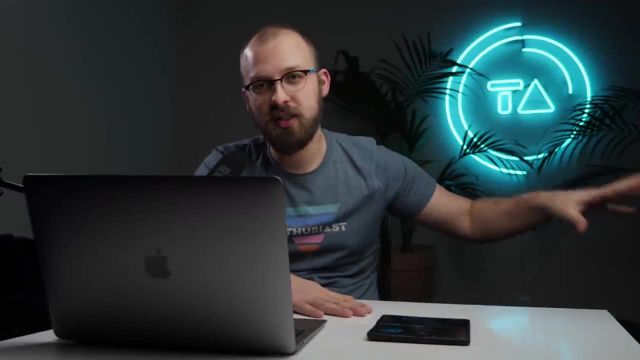 weak business, So D-tier. Let's go over to Google and the Pixel series. So I have been on record saying that I'm not a particularly big fan of the Google Pixel business, but this year they're going to go into C-tier. I would have put them into D-tier before, but I think they did. 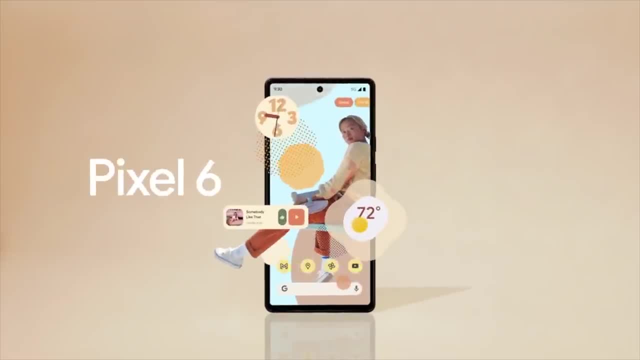 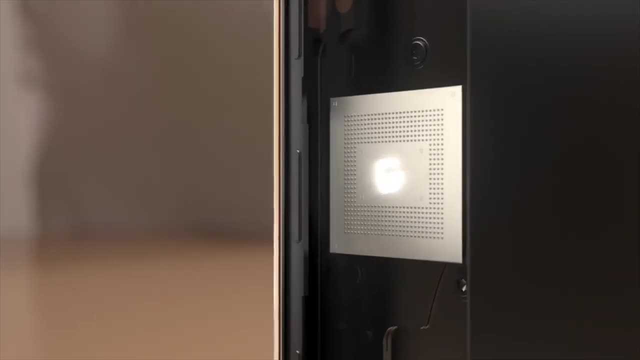 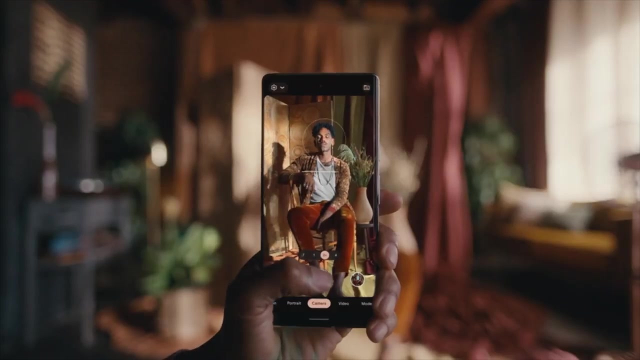 better this year than usual. I think the Pixel 6 series is their first product that is a true, unapologetic Google product. I feel like it is a proper flagship. It has its own unique design, its own unique technologies, including its own chip, its own strong AI capabilities. 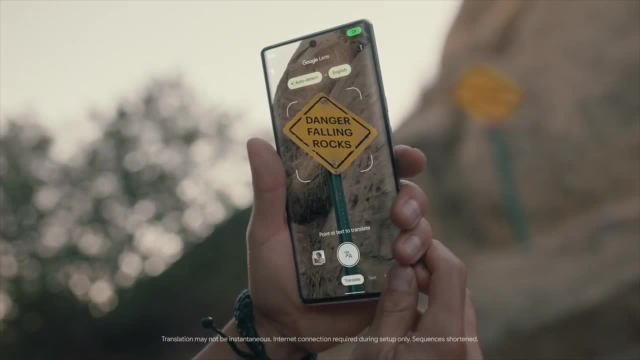 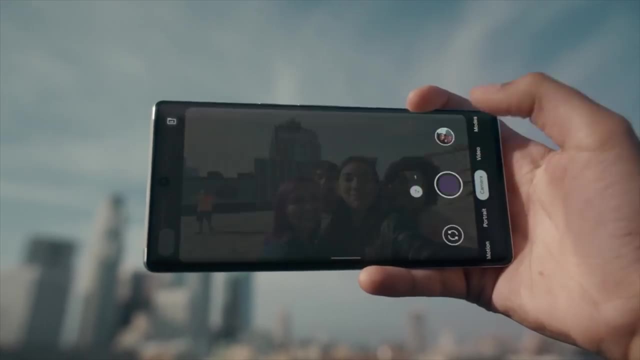 they finally put some real marketing muscle behind it as well. We don't have any sales figures from the Pixel 6 yet, but this is a solid, interesting product at least, And so I'm giving them a C-tier this year, and I hope they're going to go even higher next year. Honor. I would put Honor into the C-tier. I'm very impressed that since they have left Huawei, they were able to establish themselves basically at all. Obviously, they have built up a new business, which is a very good thing. They have a very good business, which is a very good. 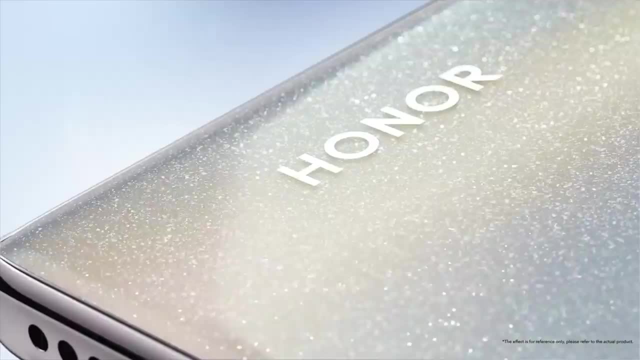 business. They have a very good business, which is a very good business. They have a very good business. They have a new device portfolio that is still very much inspired by all the things that they took from Huawei, So they're all still a bit of just Huawei phones in disguise, but they have now. 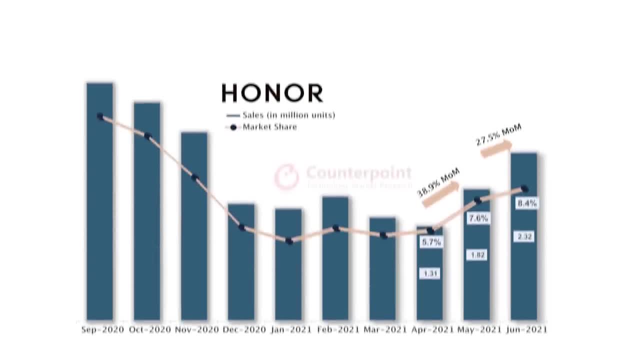 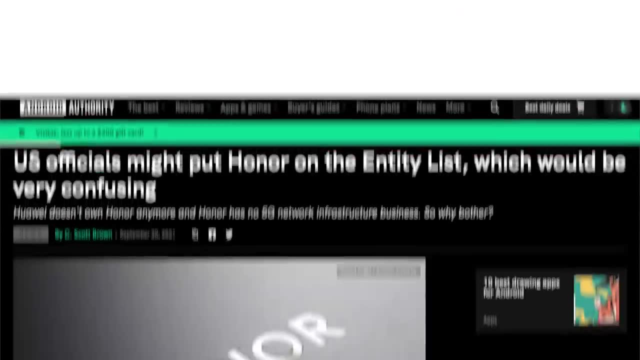 a relatively solid portfolio that they're selling both inside China and outside of China. They managed to reach, I think, the number three spot briefly in China, So they kind of clawed back a lot of their lost market share. They might be put on the anteater list by the US, so maybe. 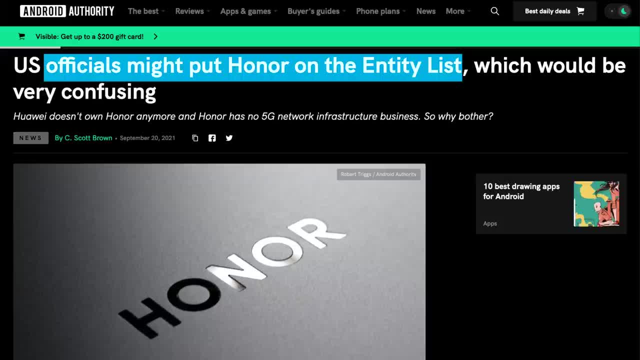 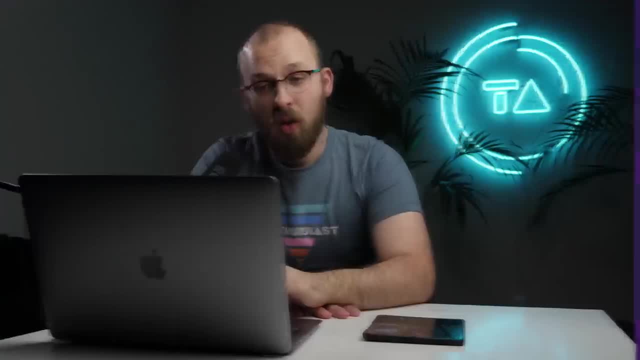 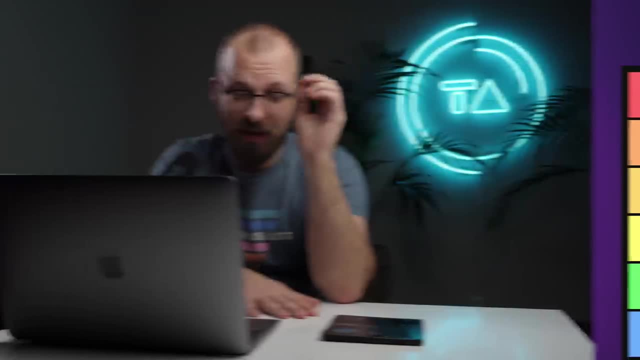 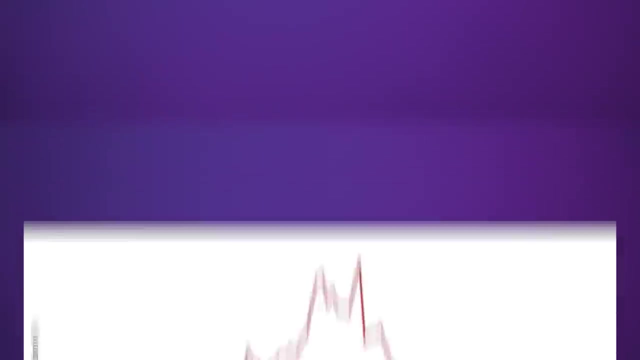 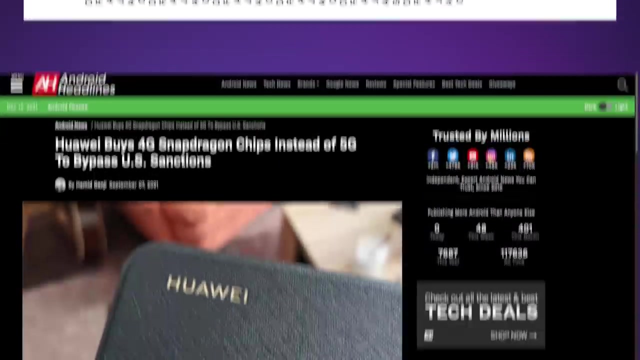 their business outlook is not as solid, but I'm just impressed. Huawei, on the other hand, in my opinion, is getting a D-tier. They're still obviously under a ton of pressure. Their international business has basically completely collapsed. I am impressed that they managed to kind of stabilize their market share. It seems like 8% in China. That is kind of impressive. I'm also impressed that they managed to make a deal with Qualcomm to have at least Snapdragon chips. 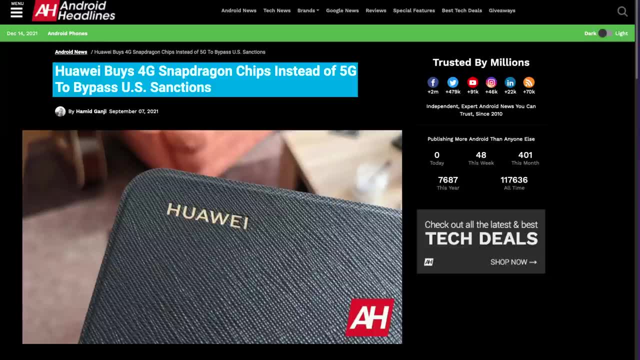 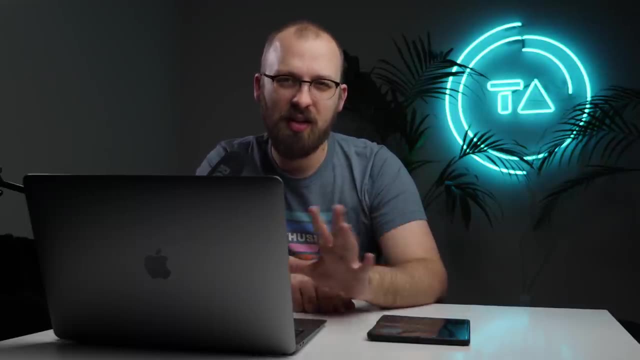 in their phones if they can't make Kirin chips anymore. But of course they can't get any 5G Snapdragon chips. China, their only last remaining market, is probably the market where 5G is the most important for consumers, So this is a very difficult position. I think their Harmony OS 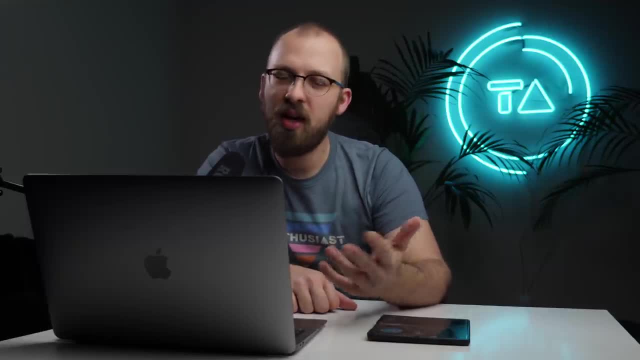 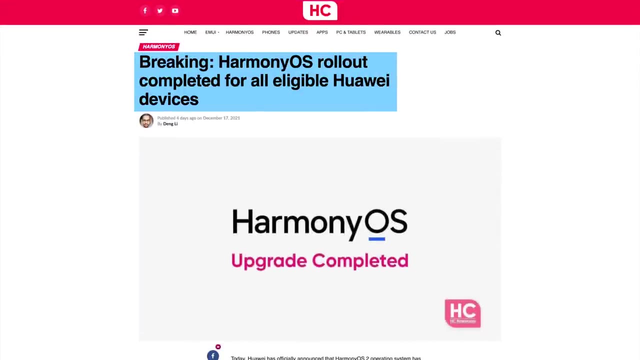 initiative is going okay. I mean, they apparently managed to roll it out to every Huawei phone that they plan to roll it out to in China, And they also managed to get a couple of other phones that they plan to roll it out to in China, And they also managed to get a couple of other. 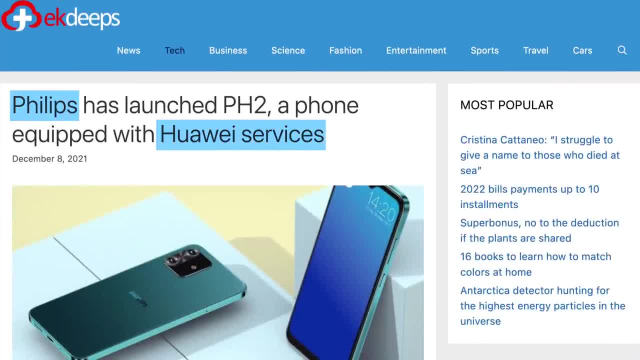 phone brands, for example Philips, a couple of these small ones to release phones with Huawei mobile services on board, And there's a couple of Harmony OS ecosystem partners. So it's not completely dead. But obviously that rollout didn't go internationally anywhere either. So 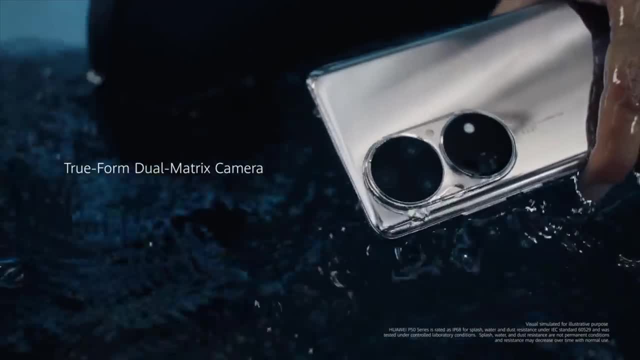 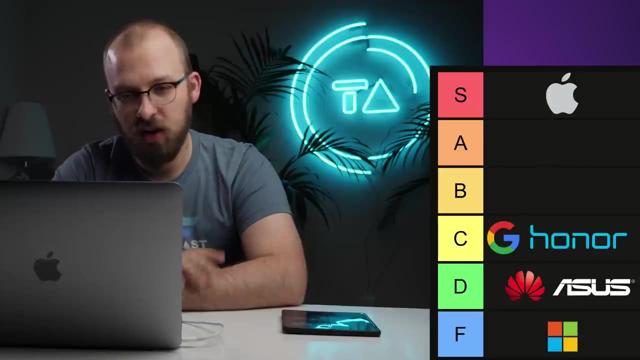 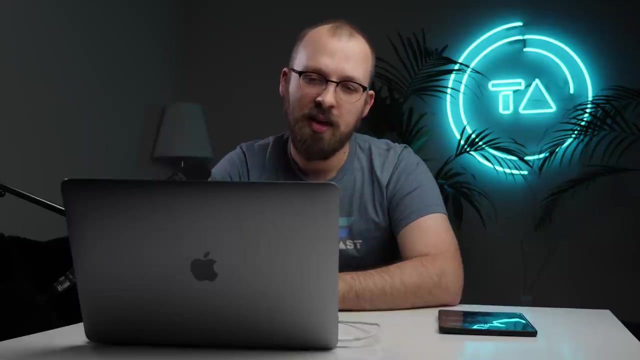 it's a very difficult position. They're doing their best, But I think the most I can give them is a D-tier. Microsoft is going to be our first company in the fail category. That's an F, I think. the dual and the duo two are both interesting devices, but they fundamentally don't make sense. 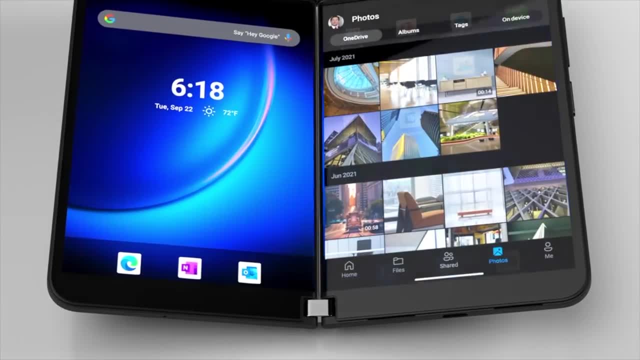 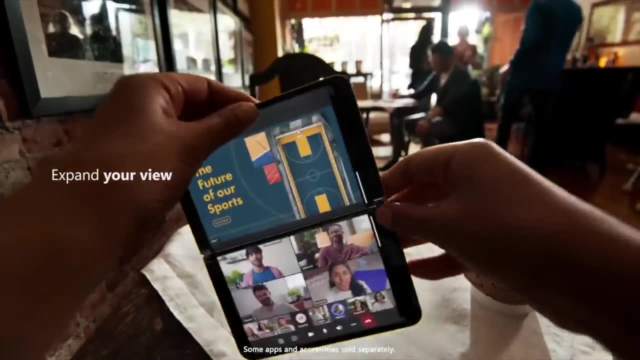 as a form factor anymore. The dual screen form factor had some supposed benefits over foldables. for example, it was supposed to be more durable. it was supposed to be have the benefit of having real glass so you can use a pen on it, and a couple of other things. I feel like the foldables. 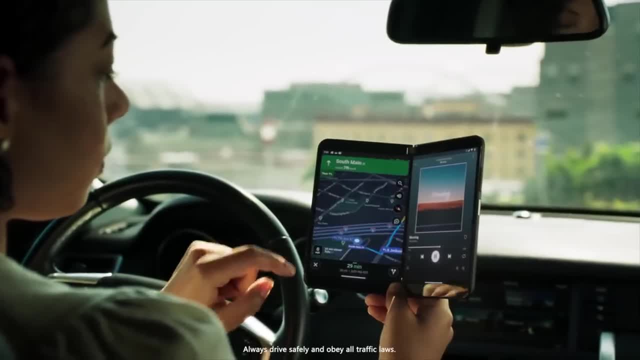 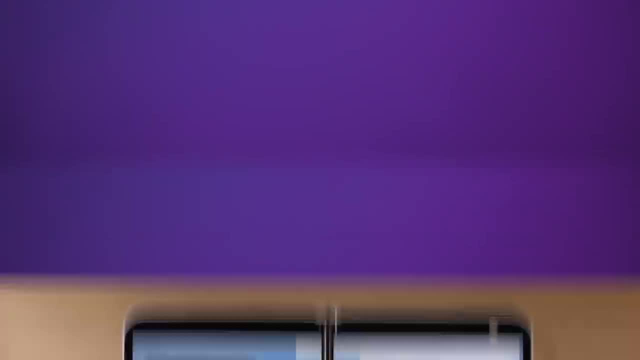 have caught up. they have overtaken the dual screen devices by now in terms of durability. For example, you can get a waterproof foldable like this when the duos are still not waterproof. Nobody is making apps for dual screen devices because nobody's buying these phones and then nobody's buying. 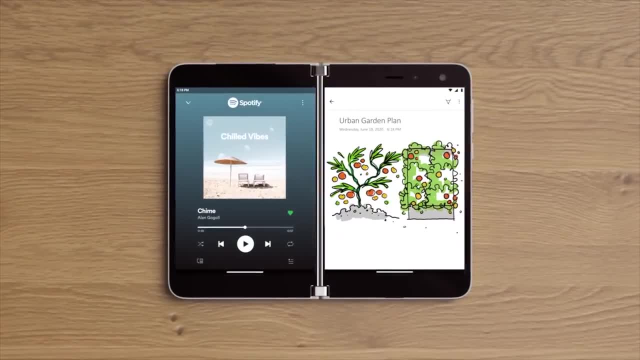 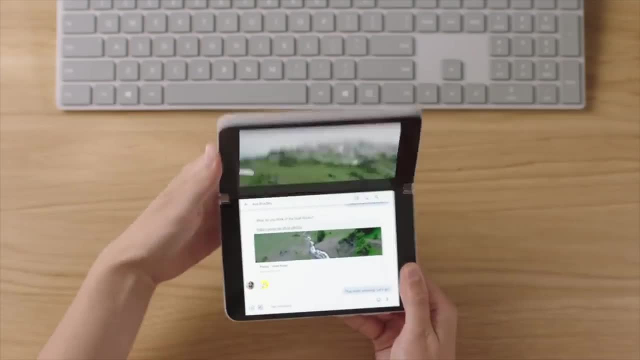 them because nobody's making them. Microsoft hasn't taken the software support of these devices seriously either, because it's such a small volume business. Apparently, the first duo, if I remember correctly, is still an Android 10.. So I feel like there might be one more try with this form factor. 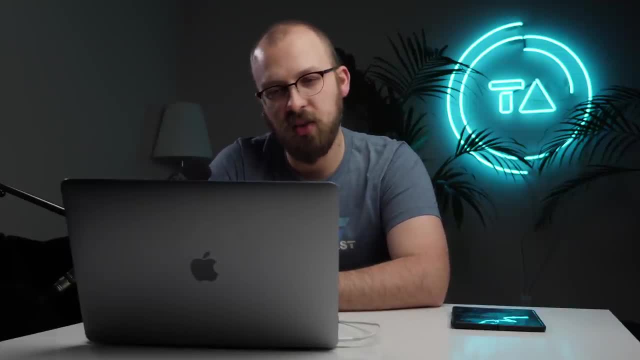 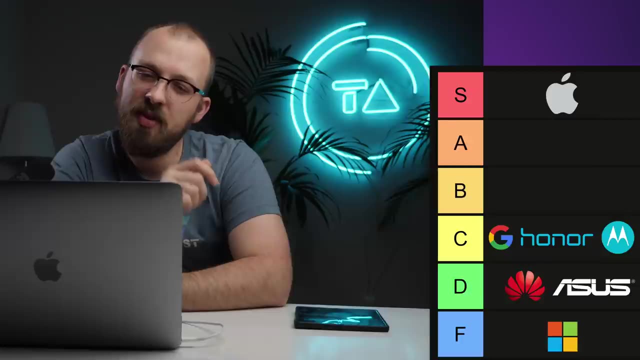 but overall I don't feel the energy behind this. I don't think this is going to go anywhere, so I think this is a fail. Motorola I am putting into the C tier and this is a brand that I would have typically put in the D tier before. I think they had a very forgettable product portfolio. 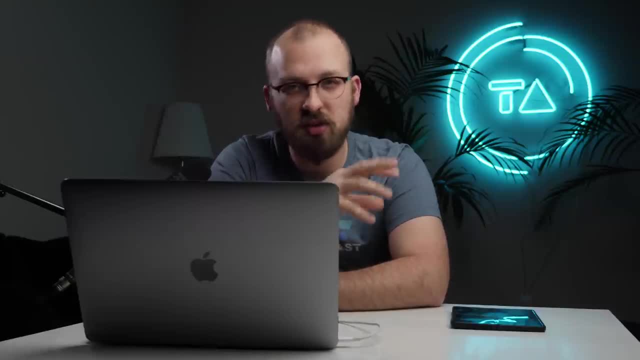 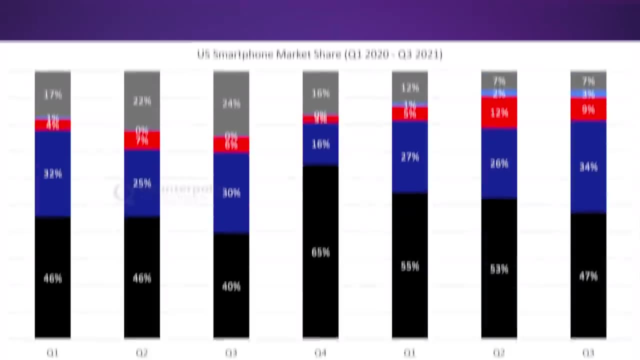 They had a pretty weak business that wasn't really growing. In fact, it was slowly shrinking and shriveling away. However, they managed to turn things around a little bit this year. In the US, Motorola was one of the biggest beneficiaries from LG pulling out of the market. 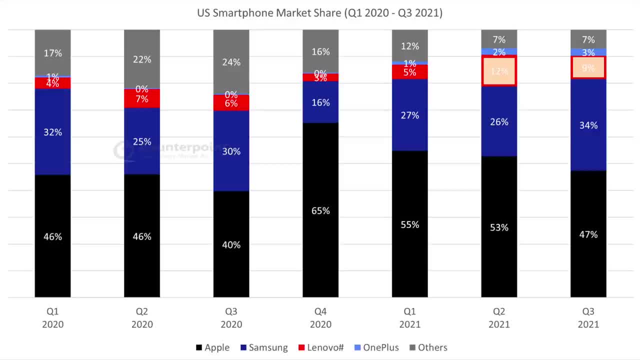 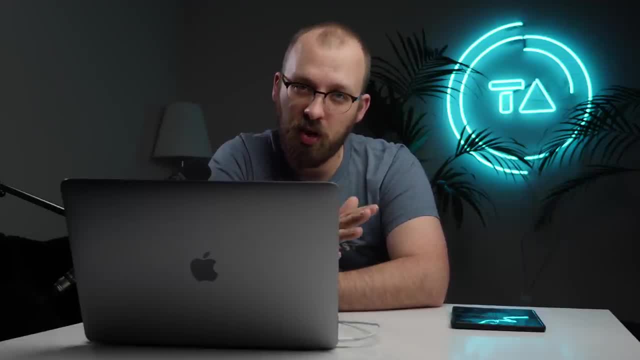 They basically captured all of their market share. They, I think, almost doubled their market share in the US, which is, of course, their biggest market. So in terms of business, they're doing relatively well. In terms of their product portfolio, I think they're also doing relatively. 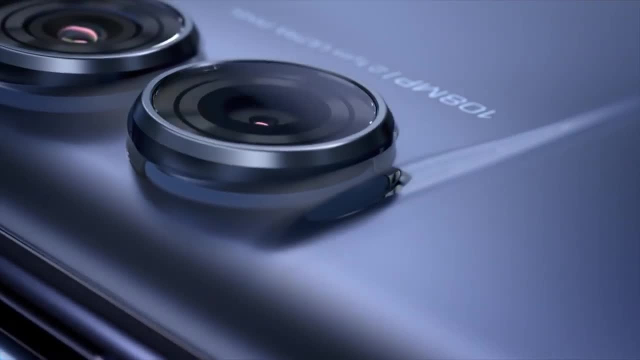 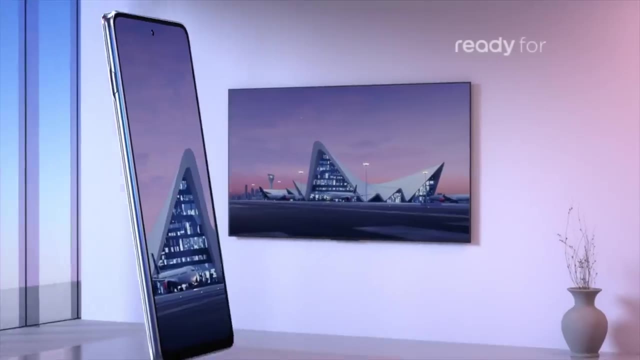 well. They managed to revamp their whole portfolio with much more aggressive prices, a somewhat consistent design language. that is, I think, reasonably good looking, And I think they have a strong market share. I think they have a strong market share. I think they have a. 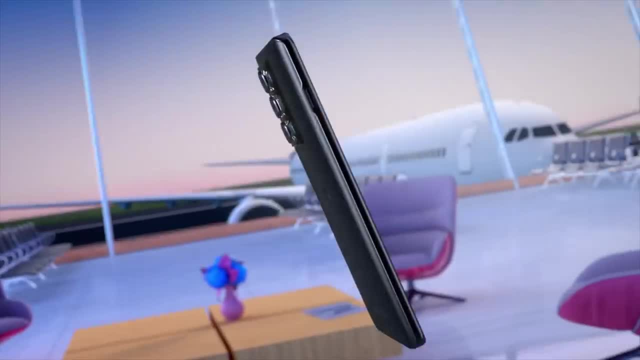 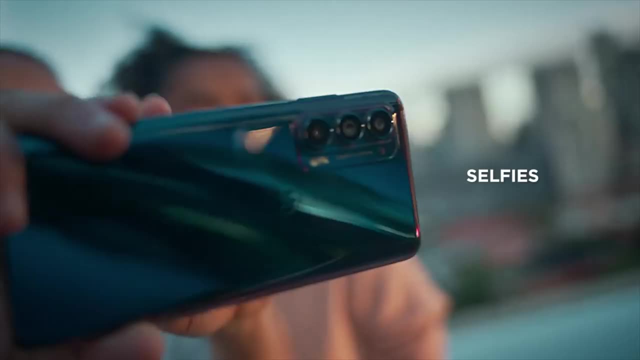 established themselves as the sort of solid device brand in the brains of many regular consumers, even if to us tech enthusiasts they're not maybe the most exciting stuff. But it's a reasonably good turnaround story that I think deserves them SC. Then we have Nokia slash HMD. 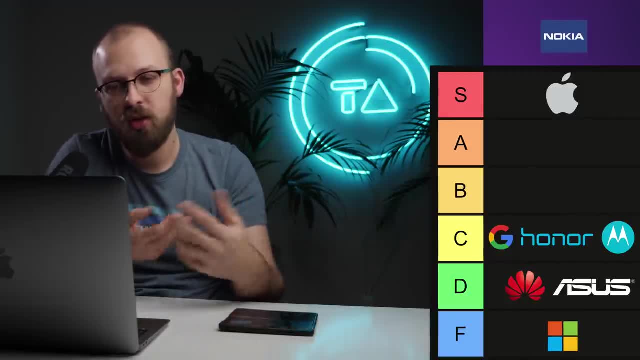 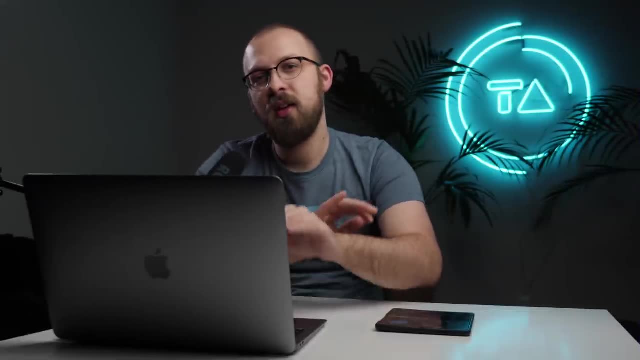 obviously the Nokia mobile brand run by the HMD company, And this is going to be another fail from me. I mean, I think they had all the right ideas in not trying to fight Xiaomi and real, me and all the other companies on price and saying, Okay, you know what? 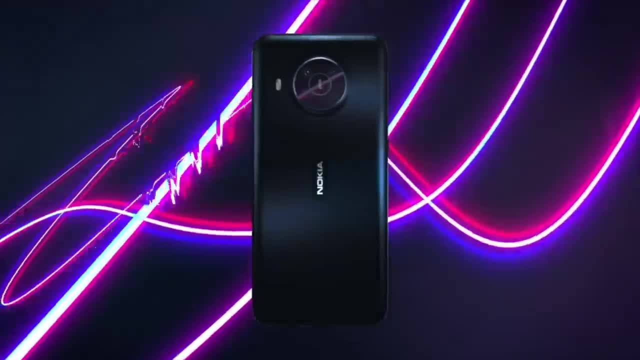 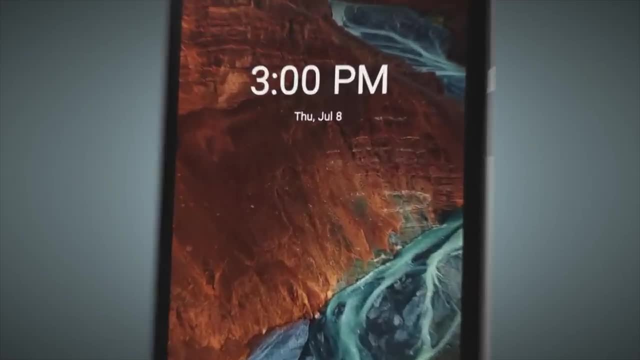 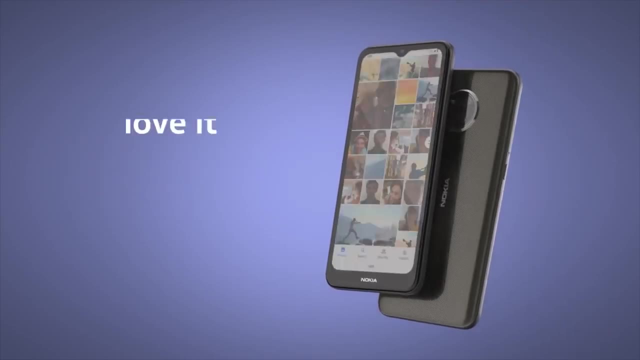 we're gonna go for something else. They said they're going to focus on sustainability, on better updates on their European Ness, on focusing on corporate customers rather than regular users and consumers, because the corporate customers care about reliability and security and all that kind of stuff more. I think this is all the right idea, But in the end, the actual 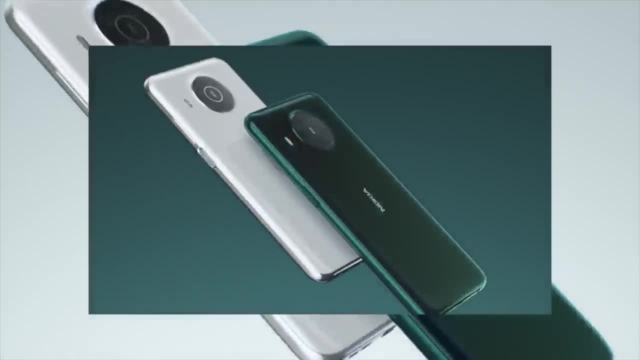 products that they brought to market. they're all super forgettable. They all look like things that are not going to work And I think they're going to focus on sustainability, on better three year old designs with the chins and the water. drop notches the prices. I don't need them. 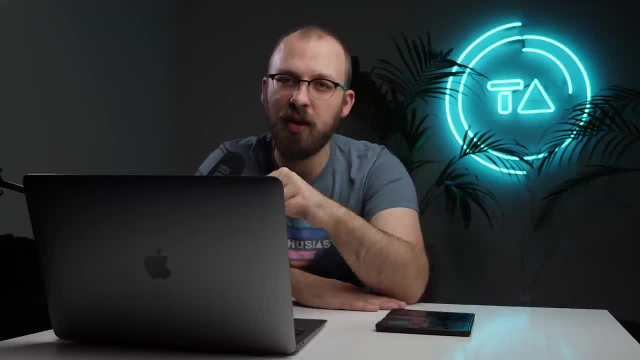 to be super competitive, But I mean the price is just so uncompetitive. In the end it's all forgettable. They had a lot of little issues like delaying or canceling updates for devices that they promised and so on, So I feel like their market share isn't going anywhere. their products. 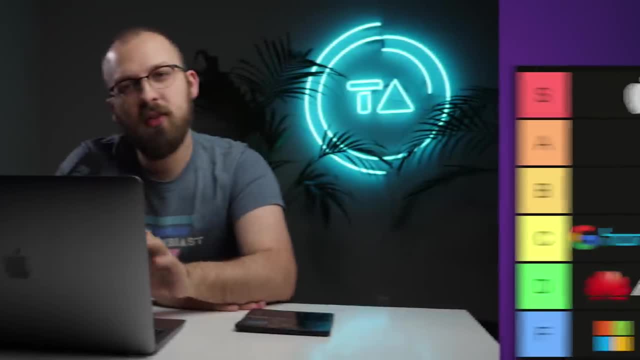 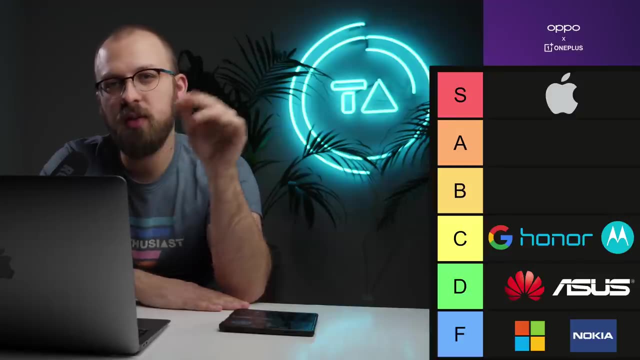 aren't going anywhere. For me, this is a fail. Then we have Oppo and OnePlus, And I'm going to be talking about these two brands. I'm going to be talking about these two brands together because the story for them this year was: 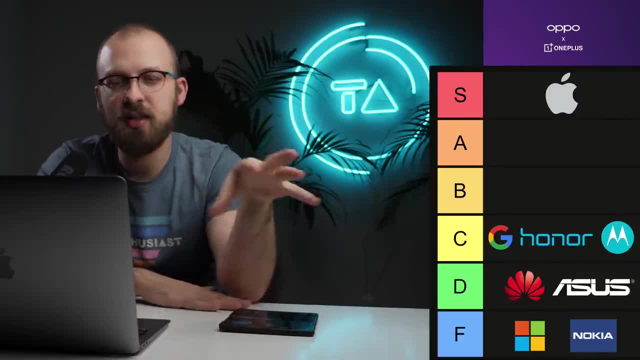 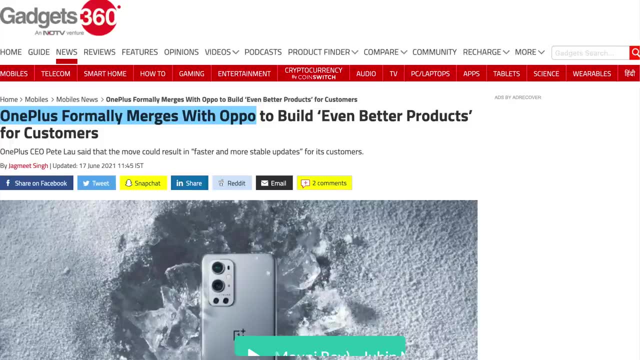 basically the merger of these two companies. That is the biggest thing that happened to them And while I think the execution on this merger was pretty messy this year, I think the idea is the correct one. That is why they're getting a, B And, of course, overall their businesses are still. 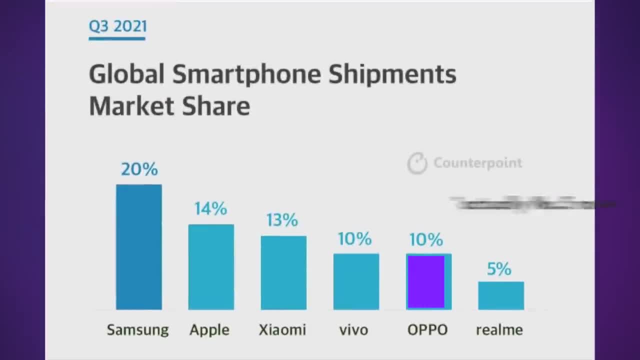 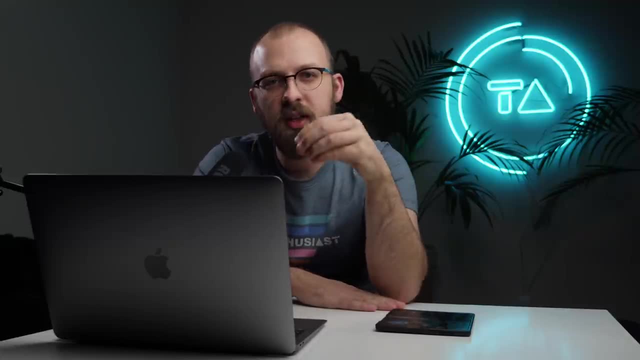 doing okay. Oppo, for example, is still the number three, number four brand in the world And overall their sales are fine. But going back to the merger, basically the opportunity for them to get a B is huge And the opportunity that Oppo and OnePlus and all these other brands are seeing is. 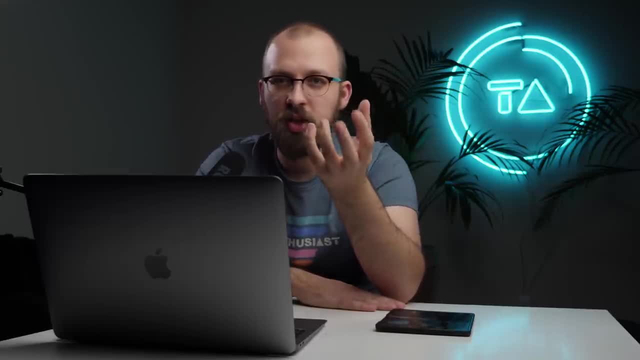 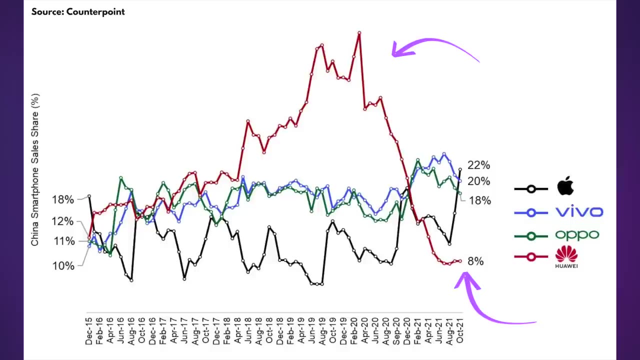 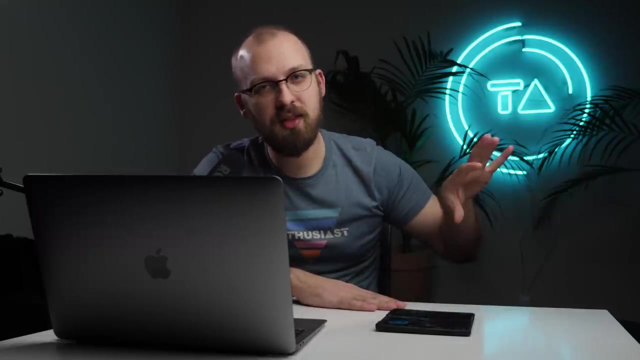 Huawei's collapse. They left a huge gaping hole in the Chinese market. They had over 40% before the collapse- 40% market share. A lot of that was premium devices And that is a massive market opportunity because with Huawei gone, the entire premium segment that isn't iOS is available and up. 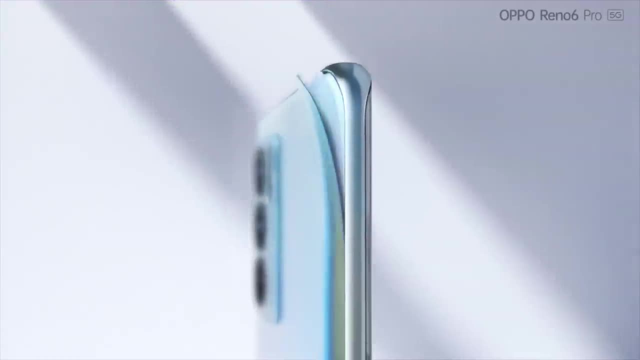 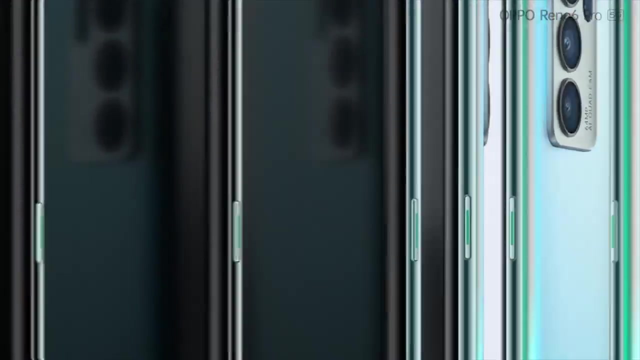 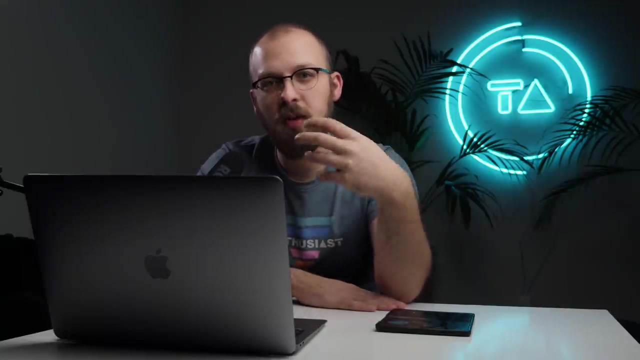 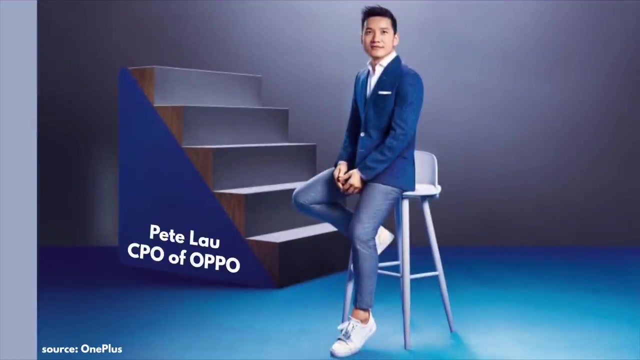 for grabs for all these brands like Oppo. So I think they're absorbing OnePlus, because OnePlus is one of the companies that have a pretty strong product DNA, a premium flagship DNA. You can see that their product people like Pete Lau are being put as the CPO, the head of product of the new Oppo. You can see new flagship devices like the: 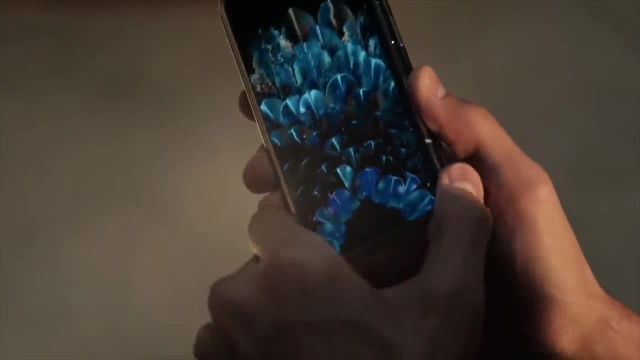 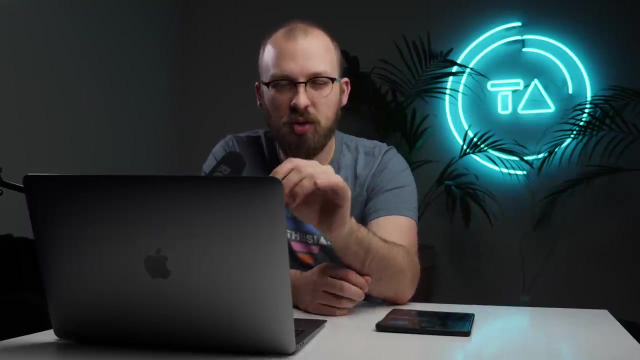 Find N being released, I think there's going to be a much heavier focus on the Oppo, I think there's going to be a much heavier focus on the Find X4 series as well, And I think Oppo is moving into the premium And I think that is the right choice. So, overall, I'm giving them a solid 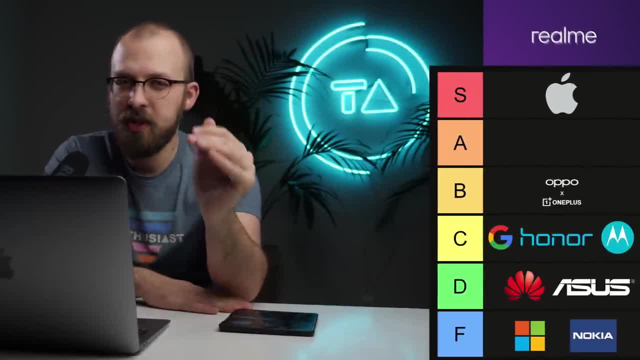 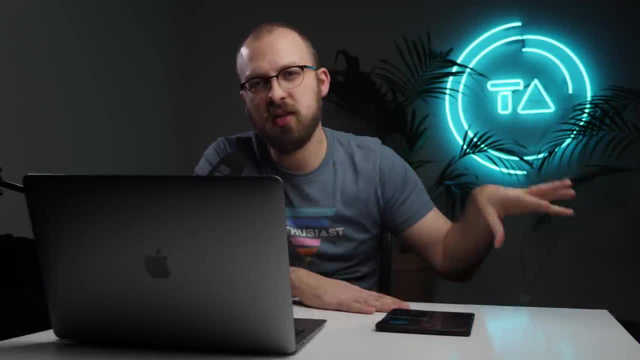 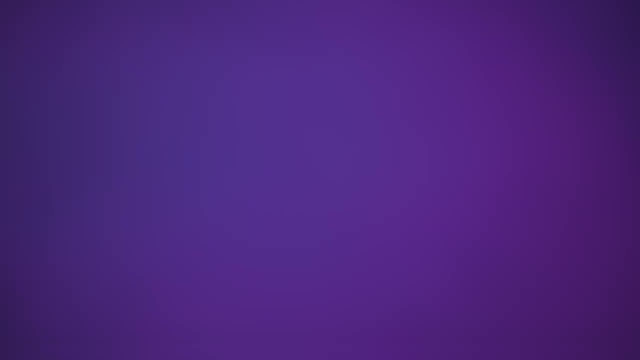 B tier. I'd say Realme is in a B tier as well. They didn't have as incredible of a performance this year as they did in the years before it. I think their meteoric rise was slowed down a little bit by Xiaomi fighting back, But still this is a solid brand. They're still growing internationally. 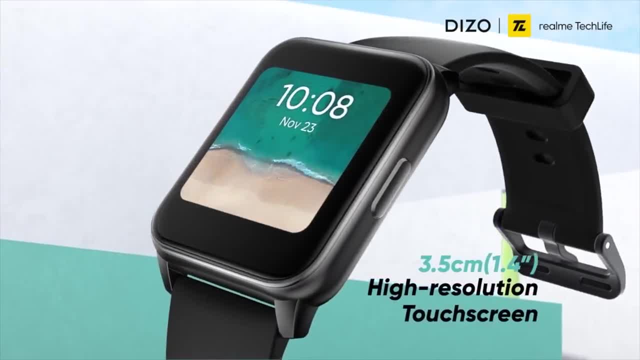 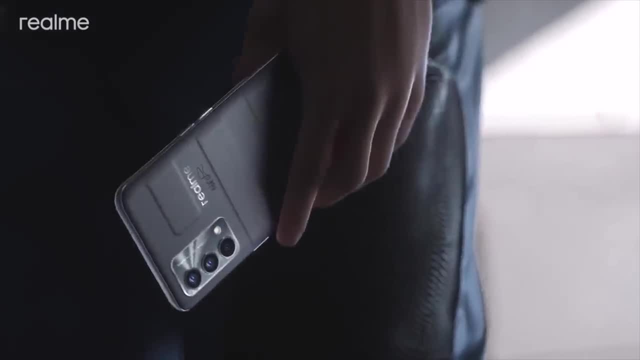 They're strong in multiple markets. They managed to copy the Xiaomi ecosystem strategy with their own Realme Tech Life ecosystem. I think they finally managed to find their own design language with the Master Series, for example. So this is a solid B tier brand overall. Then we have Samsung. 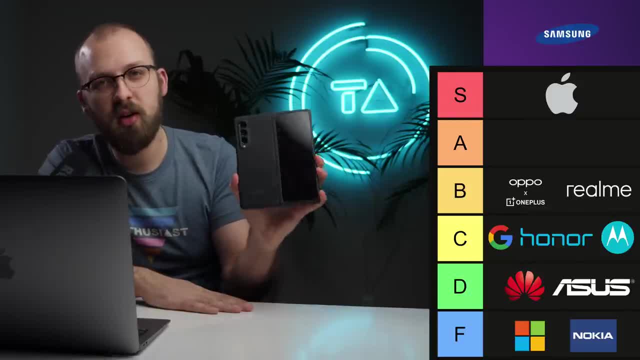 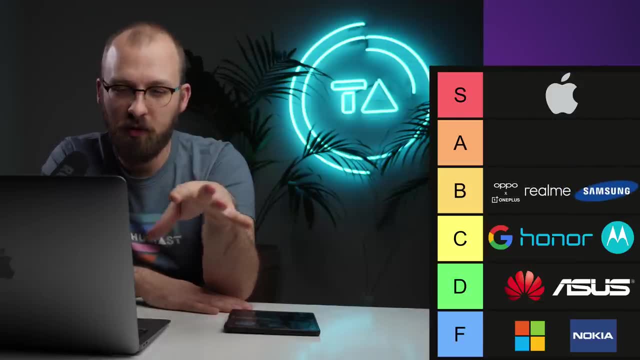 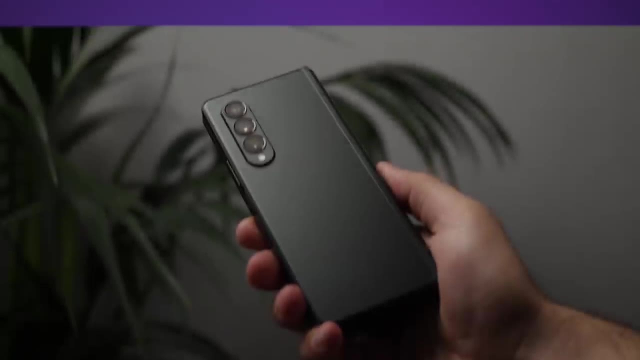 and I am obviously a big fan of their products and a lot of the stuff that they do. I think they are a top tier brand, but I think this year they're only going to get a- B from me. They have a lot of technical capabilities, a strong marketing team, a strong brand and everything. However, 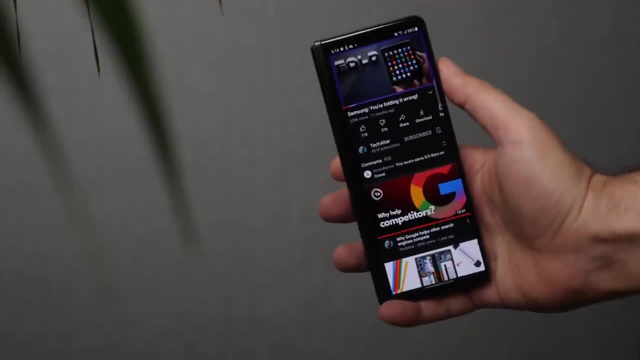 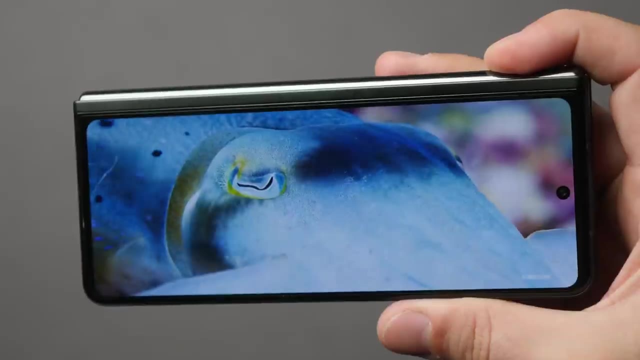 they just can't seem to be able to maintain a significant lead over the competition. All the Chinese brands that are coming after them. even when they focus on something completely new, for example the foldables- it doesn't take very long for the others to catch up with them and to 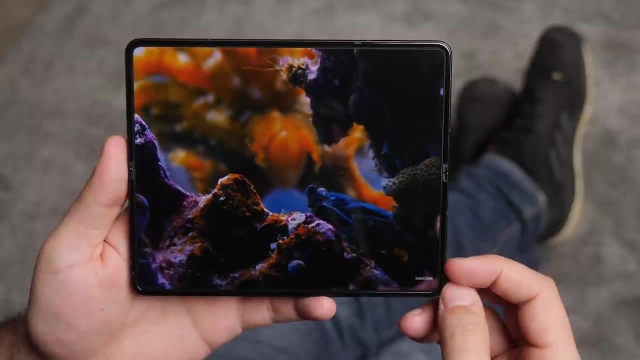 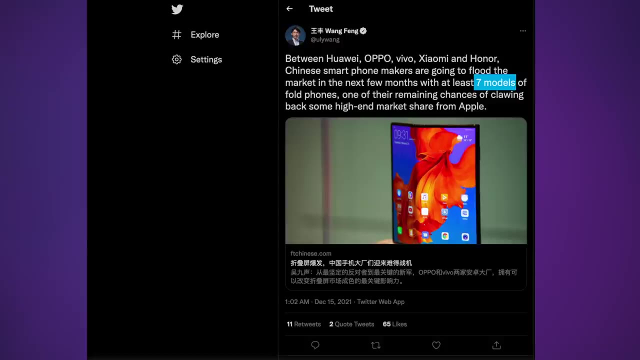 squeeze them and to press them for their margins. There are apparently going to be seven new foldable phones coming out of China in the next month or two. So even when they have the lead, it doesn't last very long. So I think it's a solid company, but just the outlook is very 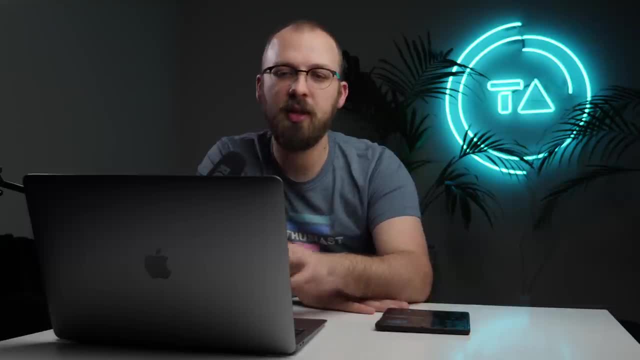 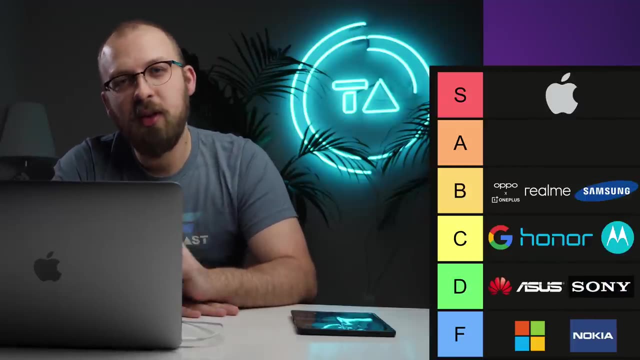 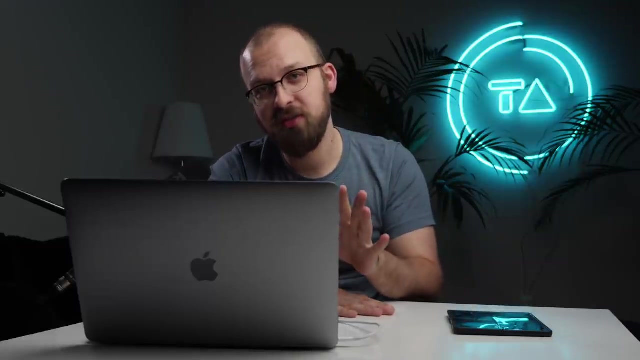 competitive for Samsung and it's going to be difficult to maintain their position. Sony, I'd put them into a D tier. Every time this company brings out a new flagship, I think, oh, maybe this is the year when they crack the code. And I think the direction, the core idea, 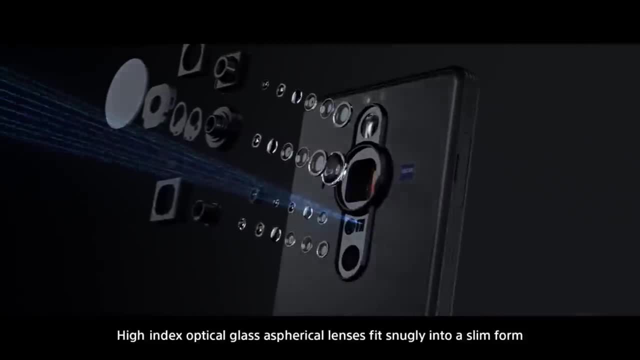 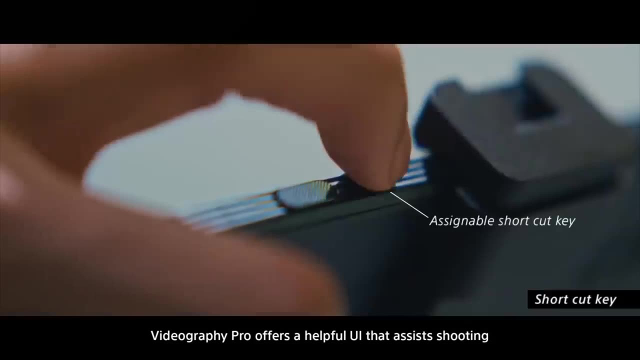 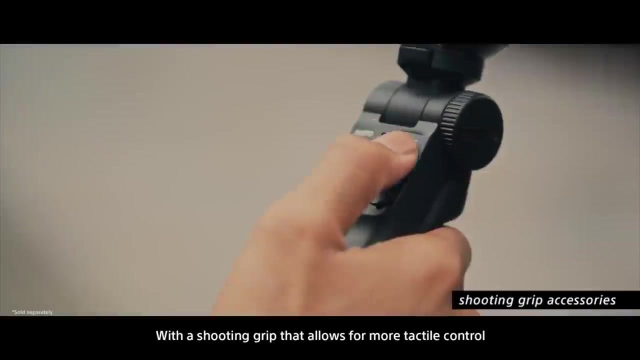 is to go into the niche, raise prices, focus on people who have a specific need from their phone, who love professional photography, who have maybe a Sony mirrorless camera. I think this is the right move And I think the Pro Eye comes closer to serving this market than any Sony phone. that. 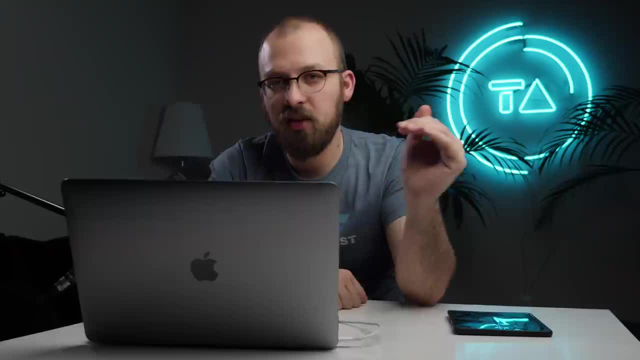 came before it in the last two, three years. Also, I'm happy that the Pro Eye availability is way better this year than previous flagships. You could buy one maybe like one month after it was announced, which is very, very good. So I think it's a good idea to go into the niche- raise prices. 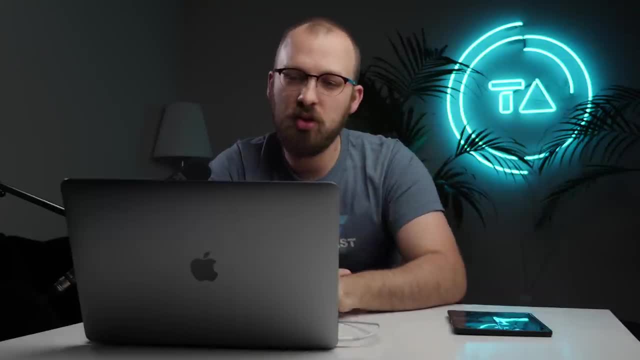 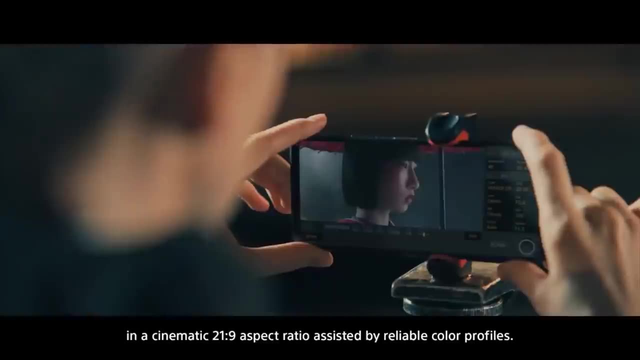 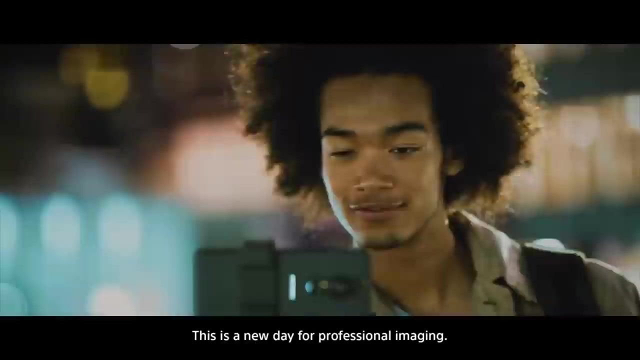 very good for a Sony phone, But generally they still don't quite manage to create a final experience that is really transcendent, that really convinces a lot of people to within this niche even to switch to Sony. So I would say it's a D generally. I hope they'll improve soon. 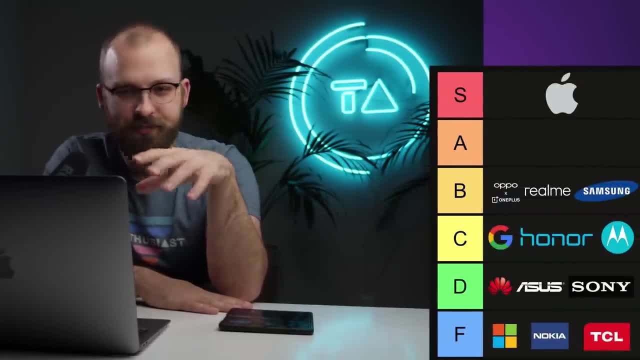 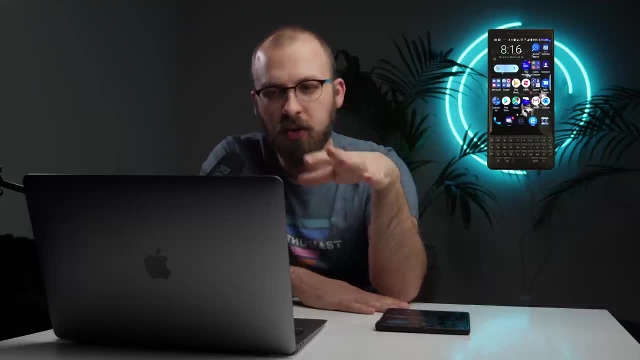 Then we have TCL, which in my opinion is a clear fail. This is a company that ran the Alcatel brand into the ground, that ran the BlackBerry brand into the ground Again. I suppose they tried to establish another sub-brand of their own. I think it was called. 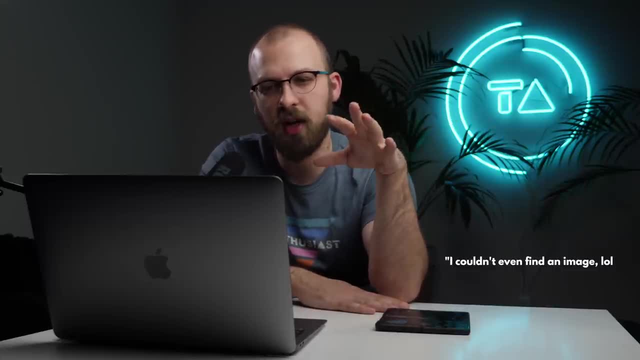 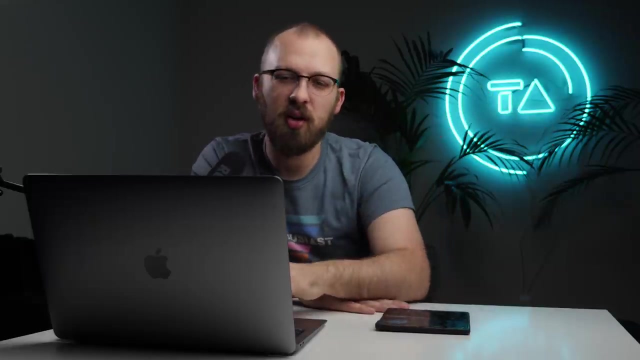 Flash. You've probably never even heard of it because that didn't work out. I mean, they had the TCL brand with new phones in the US. that was hot for like three seconds and then it faded away as well. It's just kind of a mediocre company doing a mediocre job with everything. So 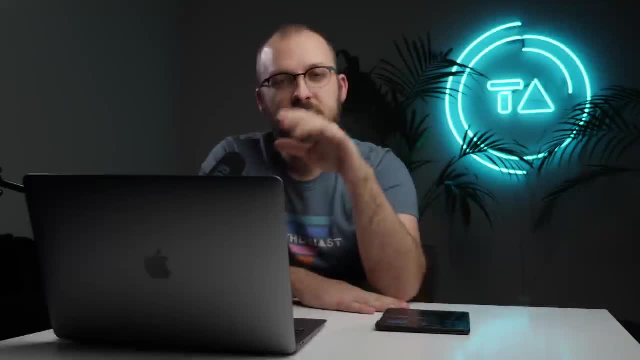 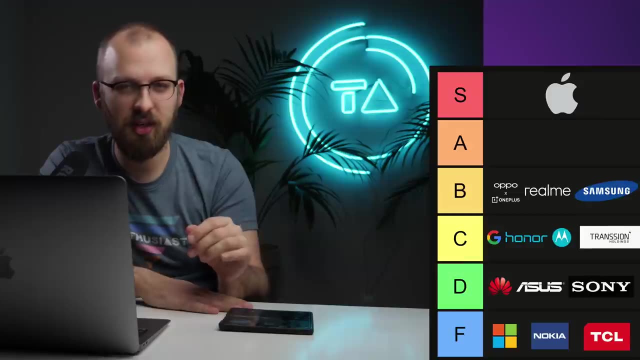 I'm not the biggest fan and it's getting a fail. Then we have a bonus company that I think most people don't know much about. It's called And it's going to the C tier, And if you haven't heard of them yet, they're basically a company. 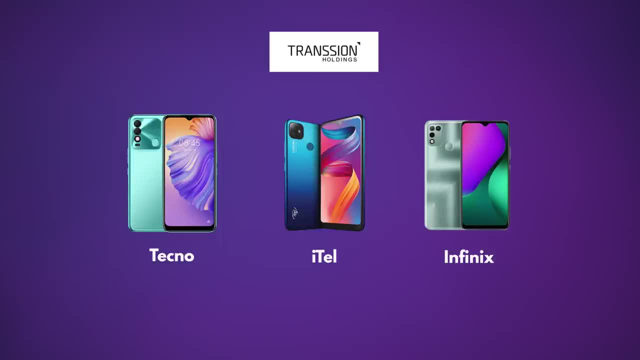 with multiple phone brands, kind of like BBK has multiple phone brands, But the brands from Transgen are called Techno and Itel, for example, and they have a different focus a little bit. So they're focused specifically on low-income countries, primarily very strong in Africa. 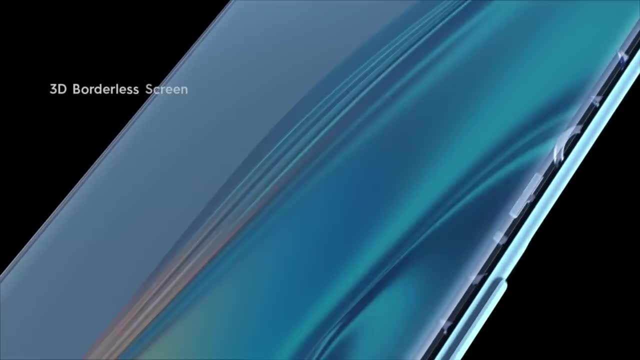 then expanding to the Middle East and to India now, And they're really growing from the bottom to pushing their own brand. So I think it's a good thing. They're way up to the premium categories. They just launched their first phone. They're a market. 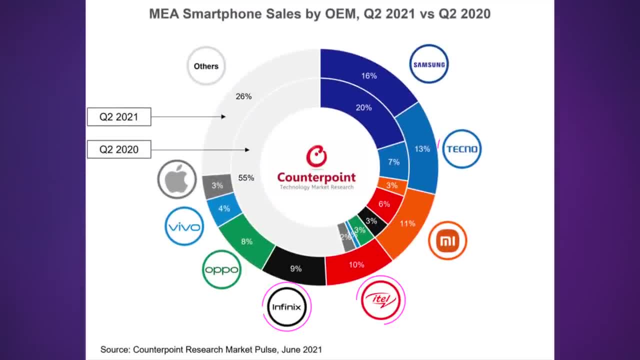 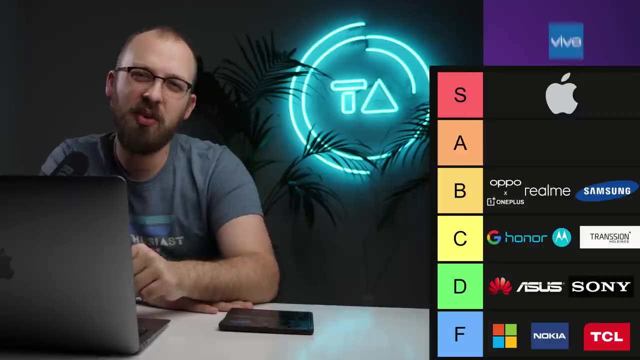 leader in a bunch of countries, like a bunch of regions, like Sub-Saharan Africa, for example. So this is a solid business with a clear strategy that is doing an okay job and their business is growing. So they're getting a C tier from me. And then we have Vivo. I'd put Vivo into a B tier. 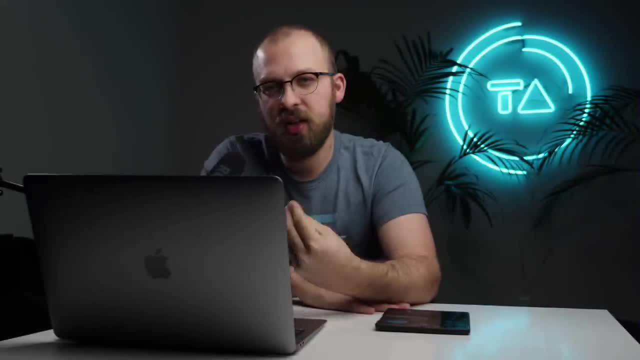 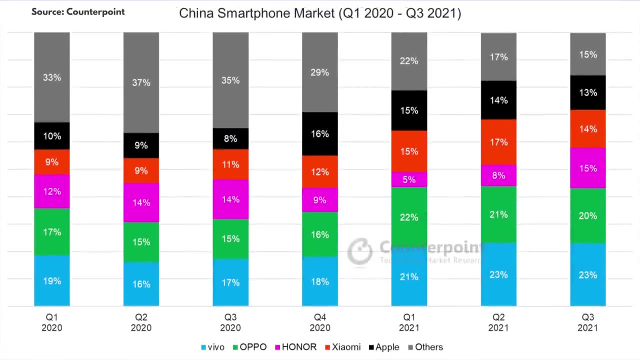 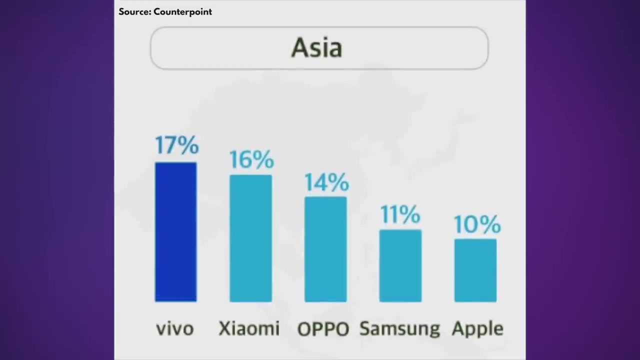 This is a brand that I personally don't find particularly exciting, but it's just a solid business that is growing and is working well. They are the market leader in China by now. They're number one there. They're also number one in Asia, if you combine all the various Asian markets. 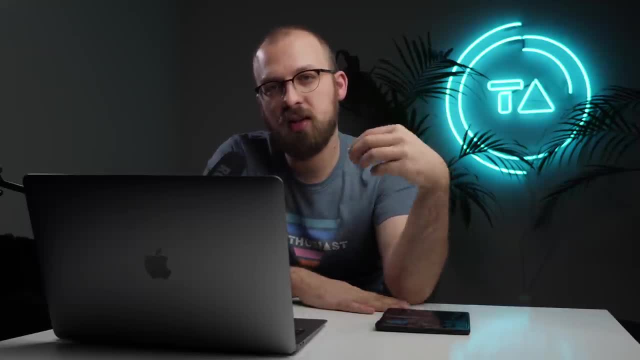 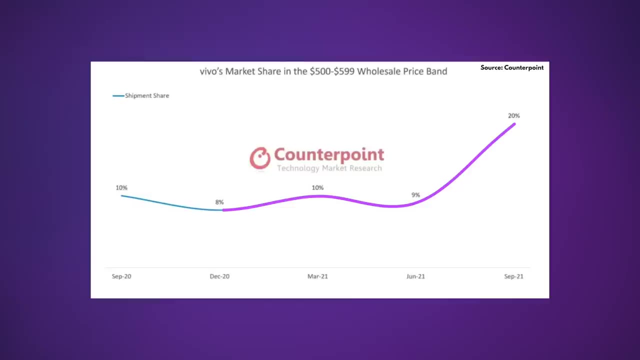 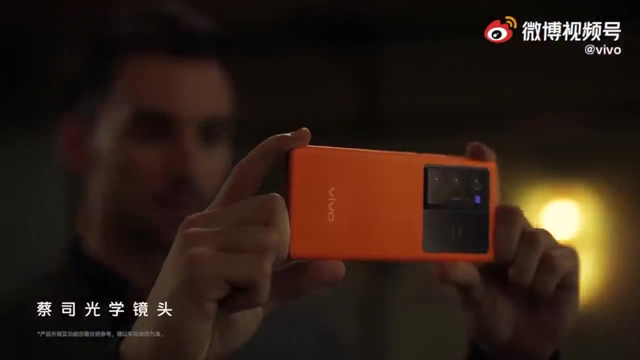 They managed to increase their share of premium devices in China from 8% to 20% in about a year, So they're moving into the space that the loss of Huawei has created. They managed to create some strong tech partnerships, for example, with brands like Zeiss for their camera. I feel like they managed to establish a strong design language for their newest flagships as well. So they're just generally a well-run business. They're efficient, Distribution is strong, Marketing is strong, Brand is strong, Products are decent- Not my favorite business, but it's. 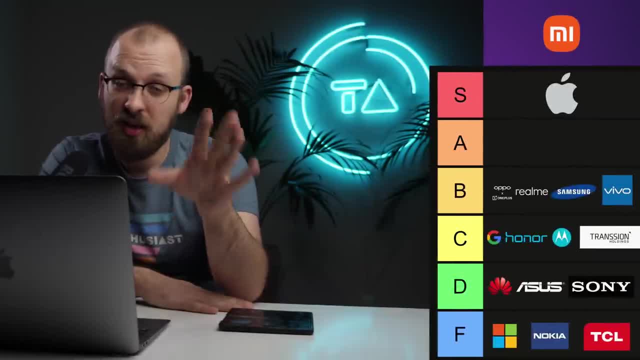 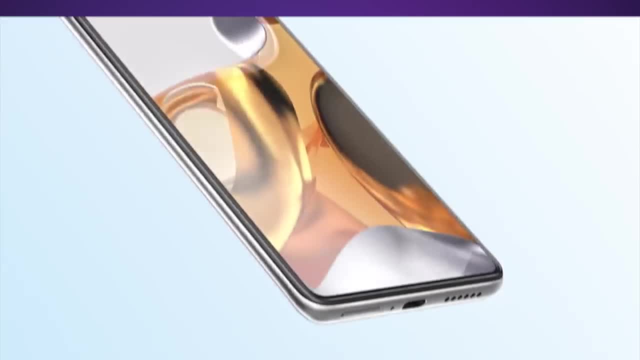 a solid B tier, I think, And the last on this list, and also the only brand that is going to get an A tier rating, is going to be Xiaomi. So they had a bit of a temporary slowdown in the last quarter. They had a bit of a slowdown in the last quarter. They had a bit of a slowdown in the. 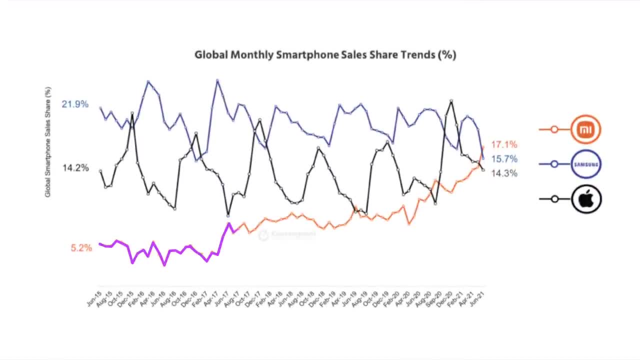 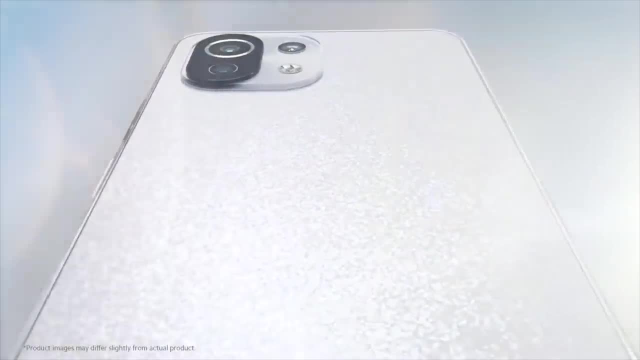 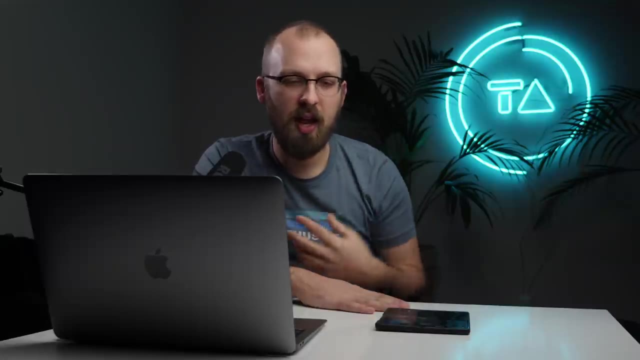 last quarter due to supply chain issues, But overall, this brand is on an incredible trajectory. They managed to prove again and again that their core strategy of selling phones at incredibly aggressive margins and then subsidizing that with sales of internet services, ads, as well as the 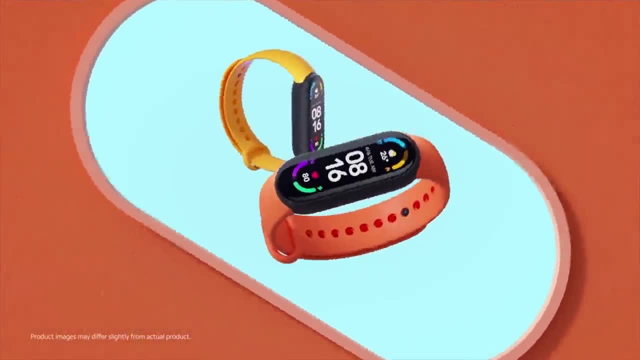 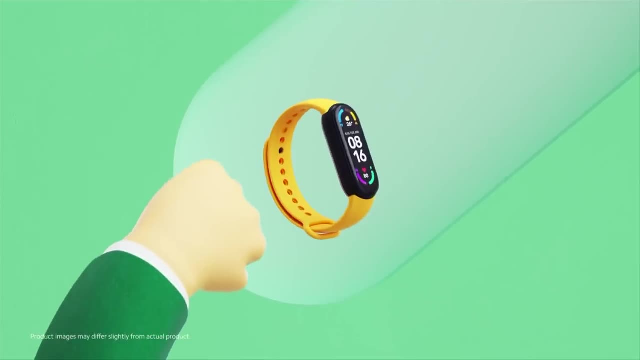 ecosystem products around: the phones, the drones, the rice cookers, the electric scooters, whatever. This is a solid strategy that works. Their execution is relentless. They're growing in all of their key markets. This is already a huge business. It's growing fast. 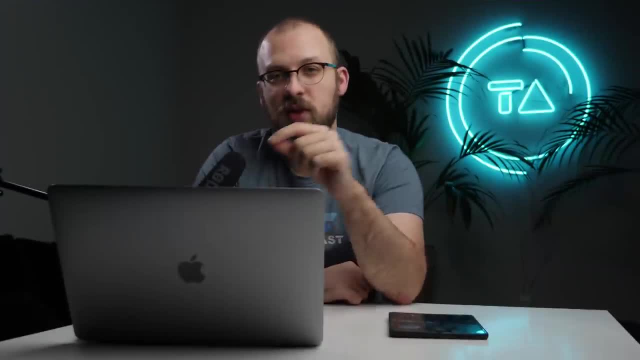 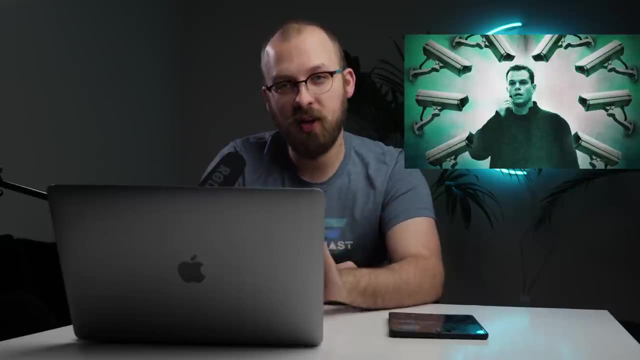 I think this deserves an A tier. All right, that's it for this tier list. I hope you enjoyed a bit of a different video And before you go, I would like to announce that we have just uploaded the final episode of season one of Technorama, my Nebula original. All four episodes are up for you to. 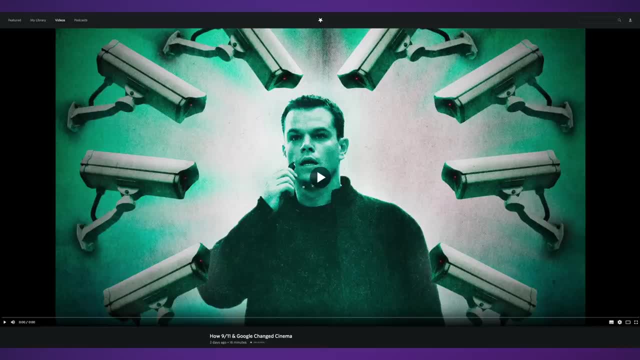 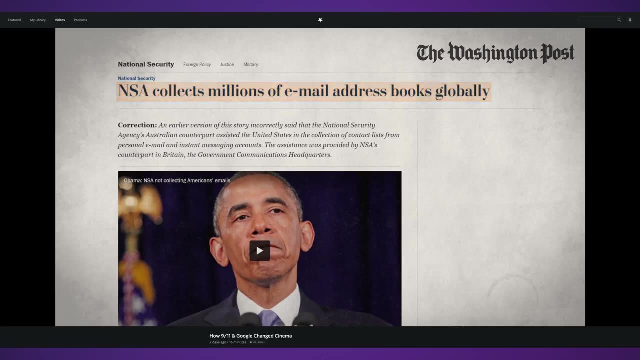 watch right now. The last one is about the different ways in which surveillance is portrayed in modern sci-fi movies, And I just want to let you know that I'm going to be uploading a new episode of this series And I just realized today that we have analyzed over a hundred different movies in season. 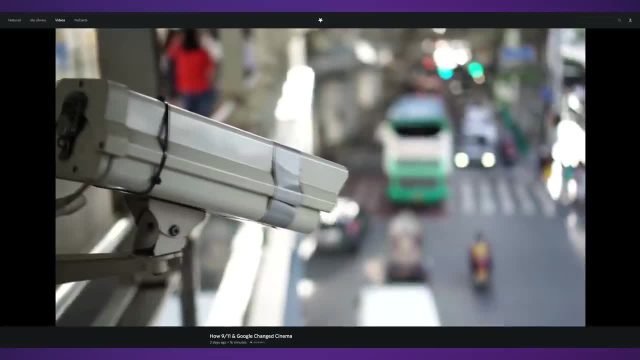 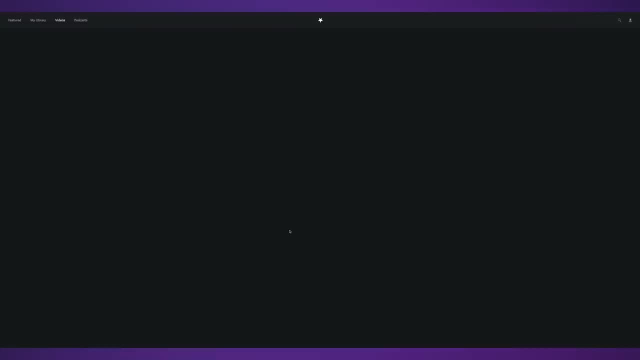 one, So if you need some inspiration regarding what to watch over the holidays, this is a great place to start. The four episodes together are about a full hour worth of film analysis. I loved making this. I hope we'll get to make a second season. I'm very happy to hear from all that have 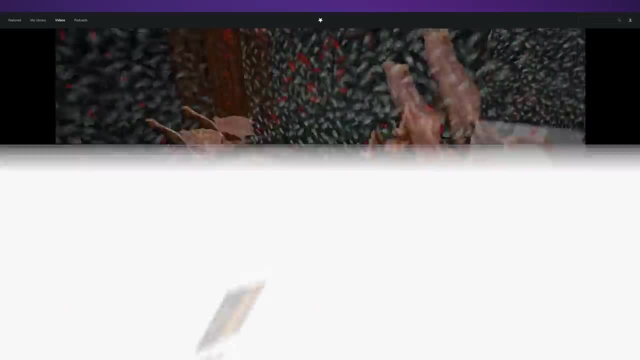 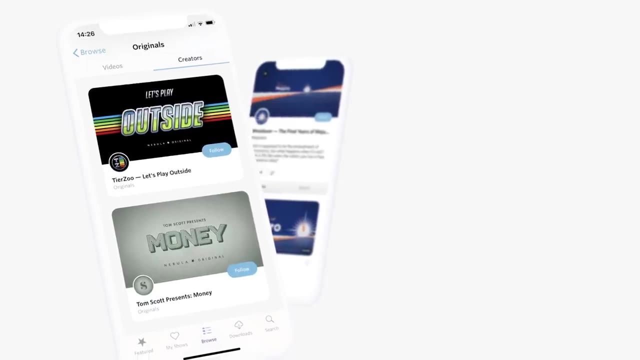 watched it, that you have really enjoyed it so far, And if you haven't seen it yet, it's time to get Nebula. Nebula is, of course, the video streaming platform built and owned by Nebula, And it's a educational creators like myself and next to full originals like Technorama. It also, of course, 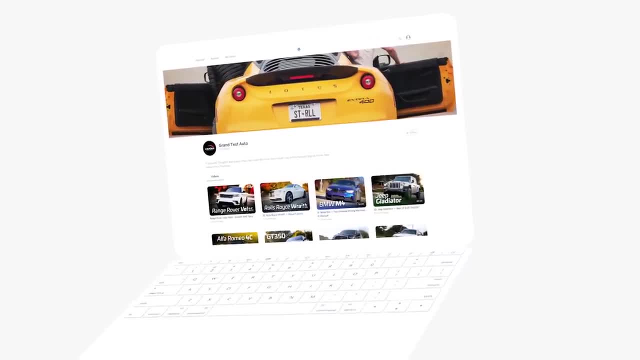 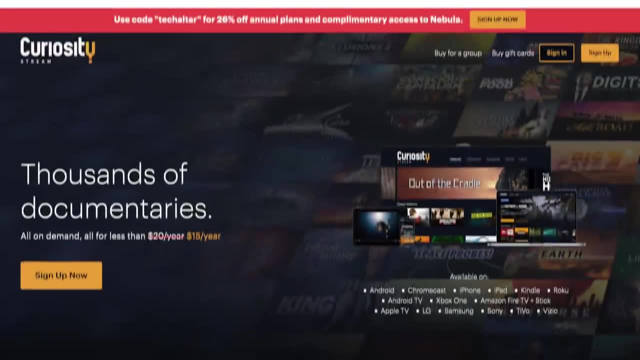 has all of our regular YouTube videos too, without ads, without tracking and often even a day or two early. The best way to get Nebula is in a bundle with CuriosityStream. That way, the two services cost only about a dollar a month for both, which is very affordable, obviously, And CuriosityStream. 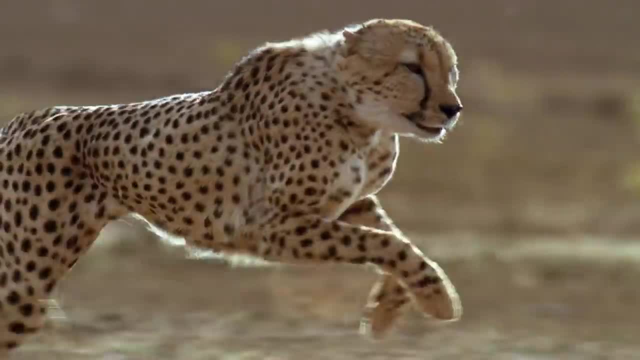 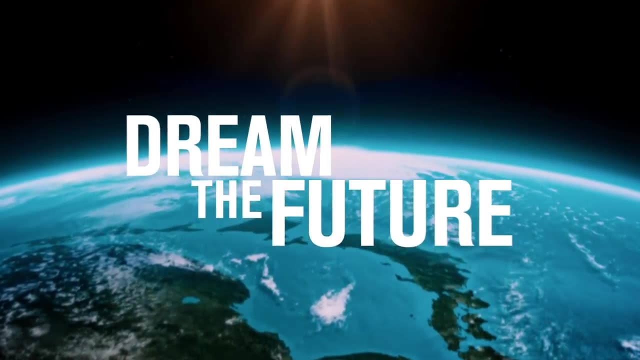 is, of course, the premier place online to watch high quality, professionally produced documentaries from history to nature, technology and more. The CuriosityStream series that I would recommend my audience from their catalog the most would be Engineering the Future. It is a great overview. 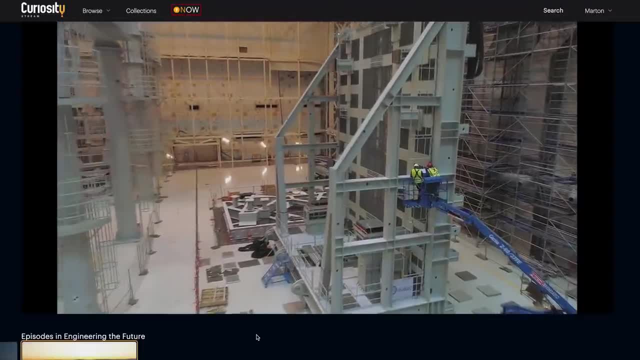 of the disruptive technologies that have the potential to shape our future. So check out the bundle at the link in the description. watch it and I'll see you in the next video.